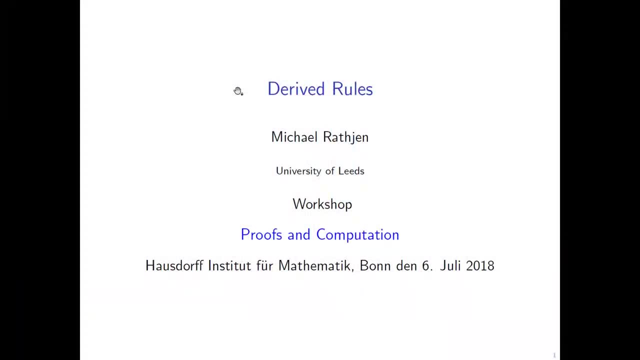 Yeah, let me thank the organizers of the workshop. I'm sorry, mind me, Right? Yeah, so the talk is in some sense it's looking back, but it's also looking forward and it's also I didn't want to talk about. 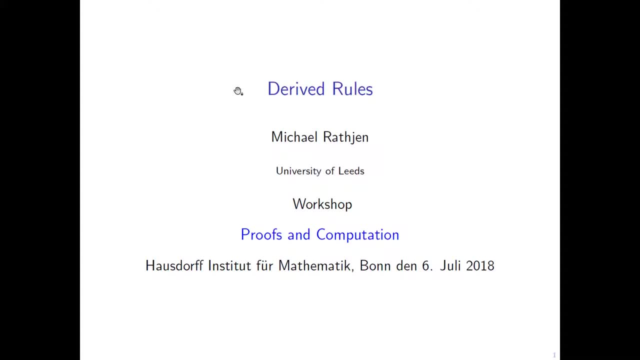 reverse mathematics because Sam was here. Okay, I can step outside if you want. Okay, so it's the derived rules. So this is something which is very special, So something very special about individualistic systems. Okay, so we know that H A has the numerical existence property. 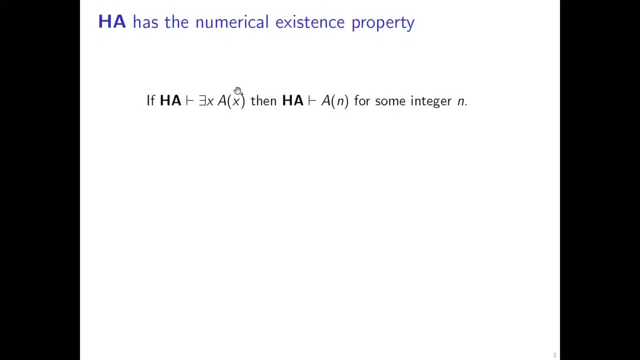 So that means that if H A proves an existential statement, then we can actually determine the integer M so that H A proves A of M. So if you look at P A, the classical counterpart, well then the two theories, they coincide, as long as you talk about statements. 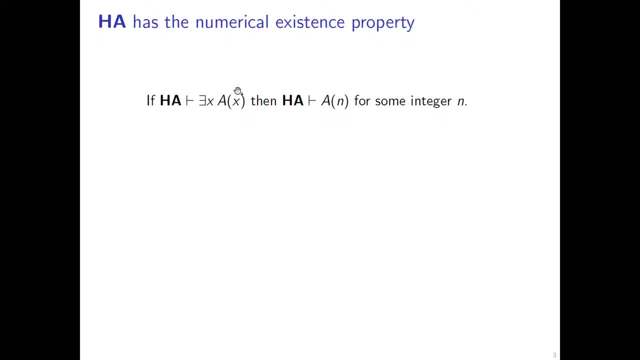 theorems not higher than pi zero two, But they diverge already at the level of sigma zero two. So here, for instance, an example. So, from the goal of complexity, so you measure the complexity of a binary string. So that's the length of the shortest input tau. 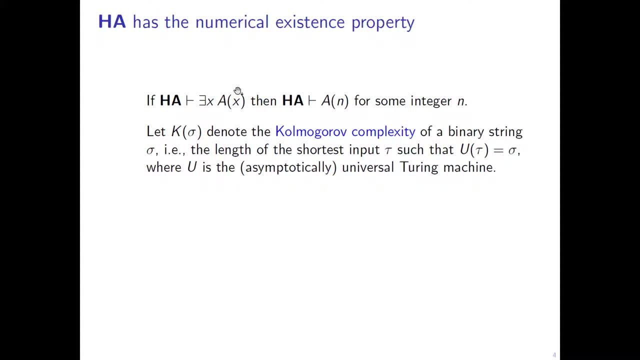 set to the universal Turing machine outputs sigma. And then in P A you can prove that for any integer M you can prove that there is a word W, so that the corner of complexity of that is bigger than M. You can actually move the quantifier inside. 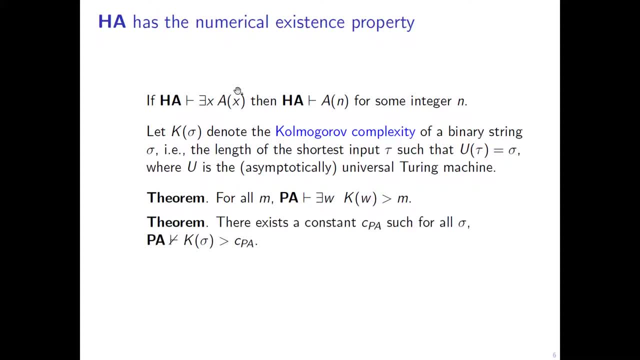 maybe beyond the term star. And then there's also- so Chaitian had this idea- that maybe these kind of that you can actually cook up certain constants so that in this case a constant C sub P A, such that if you give a binary word, sigma externally. 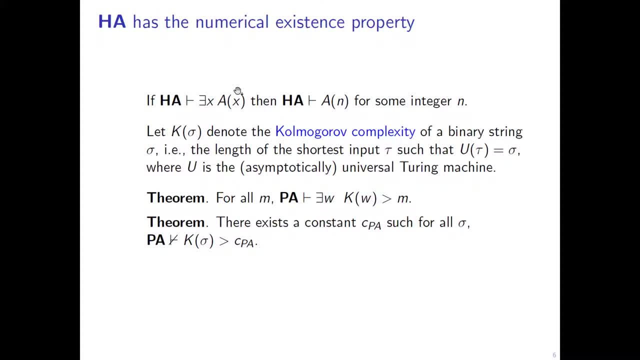 then P A cannot prove that K sigma is bigger than C sub P A. And so Chaitian argued that, argued that somehow these constants measure somehow the information content of theories. Okay, so the connection is here that, well, because of the existence property, 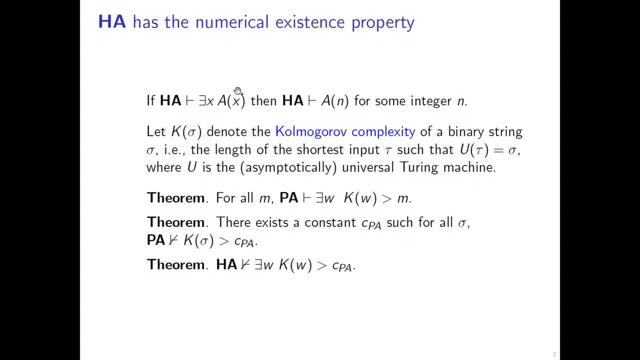 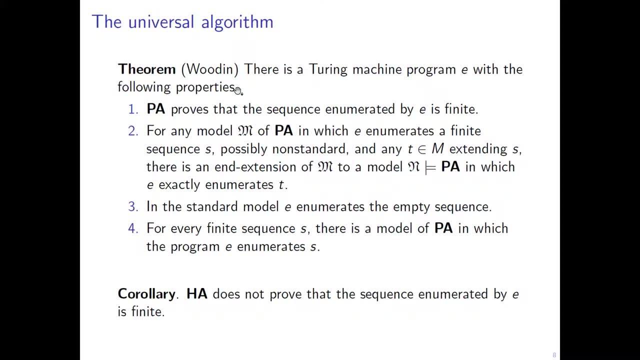 the numerical existence property H A cannot prove such a thing. So the statement of the theorem is not proved in H A. And a similar example that recently came up is this theorem of Wooden's that there is a Turing machine, program B, which has 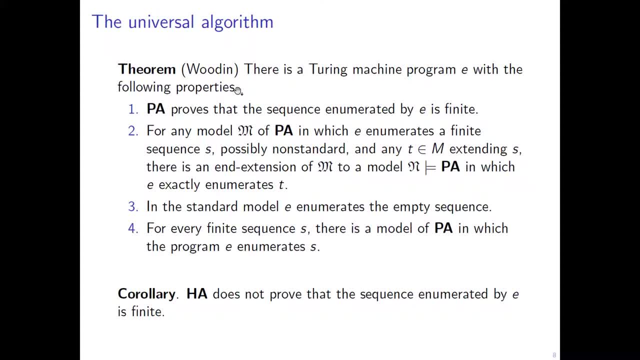 well, so that the Turing machine will enumerate which has produced output. and the output could be, of course, could produce a very long, infinite output, or could produce no output, or could produce just a finite output. And so so the theorem says that 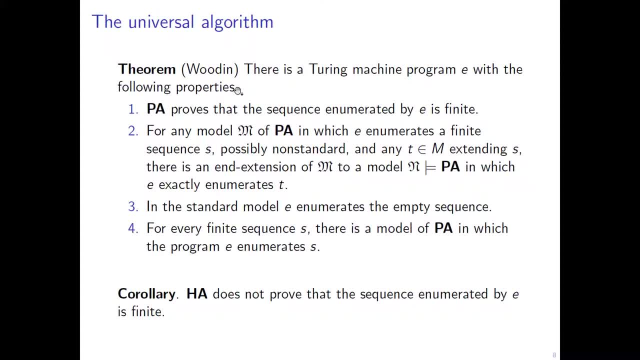 that one can find the program of the Turing machine E, so that P A proves that the sequence enumerated by E is finite. But then this has very strange additional properties And basically what happens is that in any you can't given any finite sequence, 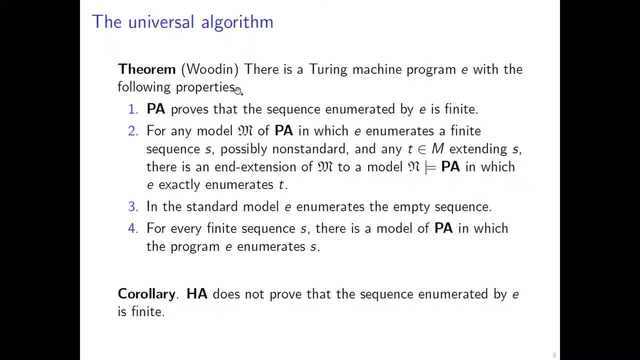 you can basically find a model of P A- usually a non-standard model- in which this finite sequence is outputted, In which this finite sequence is produced And okay, And so so this statement one, so this statement here, cannot be proved in H A. 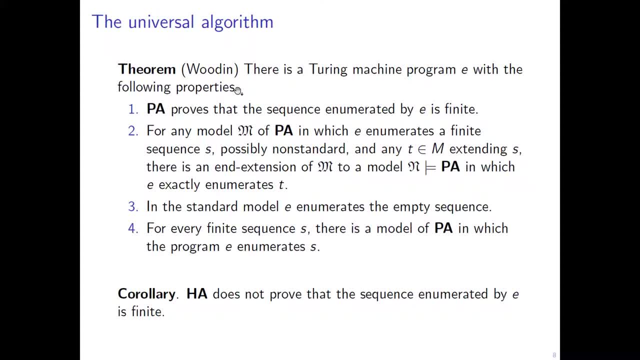 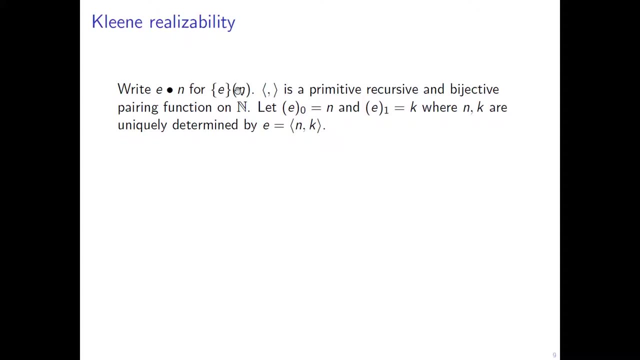 So I just mentioned this because people have made philosophical remarks about this situation, about determinacy and free will and so on, and what does it mean that they cannot prove this in their constructive systems? Okay, now to something more serious. Okay, so one of the 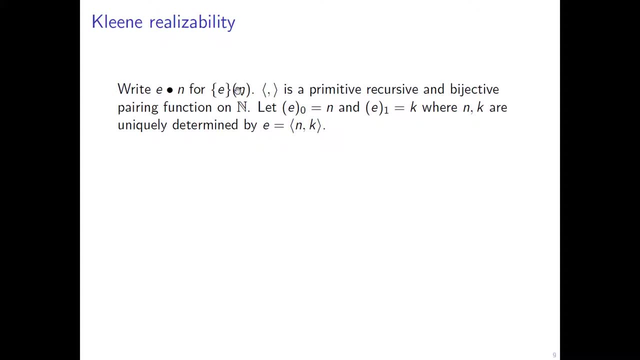 properties is the numerical existence property, and this is very, very ubiquitous. Almost all intuitionistic systems that we consider have this property, And there are many different techniques for proving this, And so one of the techniques is realisability. Okay, so we have. 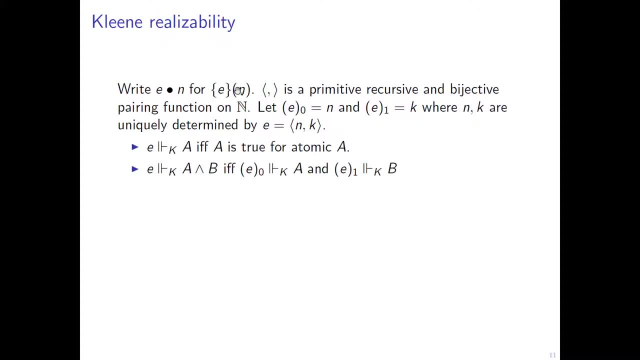 this usual clean realisability that we have seen many times here, And so, in particular, I just want to point out one thing: that these realisability- the usual clean realisability, where we use programs and Turing machines as realisers- 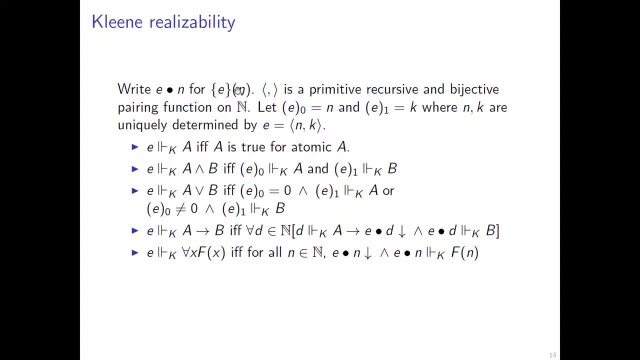 that a realisor for a universally quantified statement interacts with the quantifier. Namely, it means that for every n e of n e applied to n, so that one applies the program e to the input, n gives you a realisable. 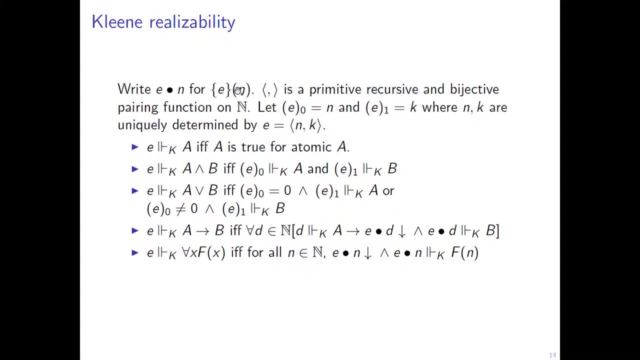 for f of n. I will show you another realisability. where this does not happen, where the realisers do not interact with the quantifiers, It's some kind of generic Okay. and so in this example, where the, where one has an application, 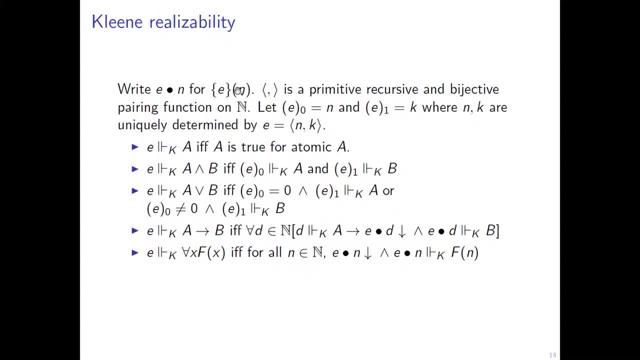 here e applied to n, so the Turing machine, e is applied to n. this means that one has some kind of domain of computation And this notion of realisability actually can be generalised considerably, basically to any domain over which one has. 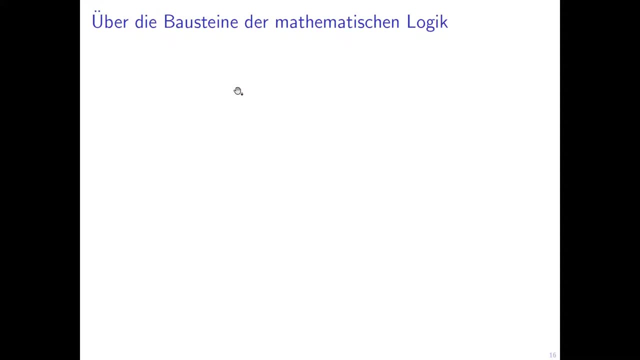 some notion of computation, And so this leads to the notion of partial combinatorial algebra. It was first identified by Schoenfinkel in the 1920s. So he had this paper about the all-style and their mathematics and logics of the basic building blocks of 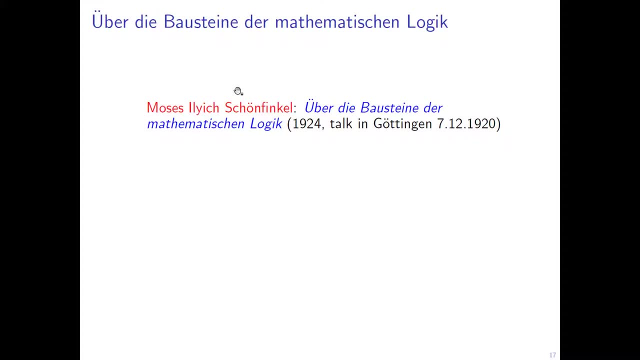 mathematical logic And this basically built actually these building blocks of building blocks of human thought, basically Something like a- I think it's a Kantorian synthetic a priori what he was describing here, And so there are some basic operations which we need for science. 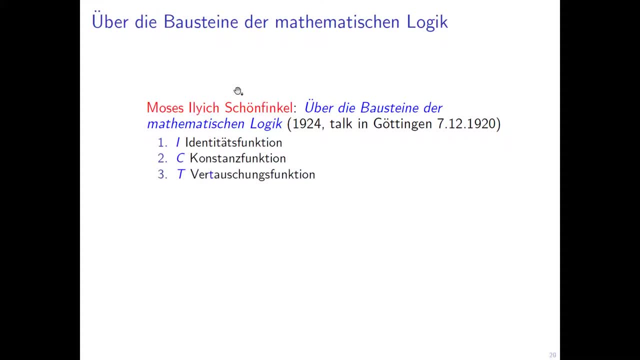 but actually for thinking. And so he had these kind of basic functions: Identity, a constant function, a Fartosian exchange, and then S, So some. I think somebody asked me about S, So why is one of the combinators called S? 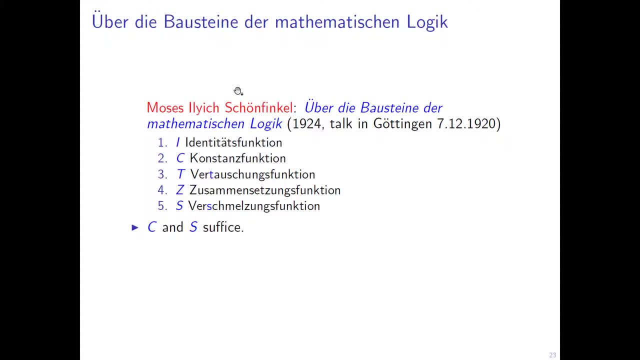 And I think the reason is that it's the German word for Schmelzl, So this kind of Schmelzl which means could be different things, but it could mean amalgamate or blend, and that kind of stuff. I think that's where it comes from. 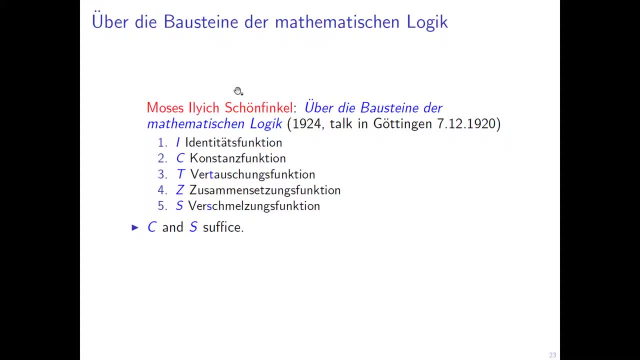 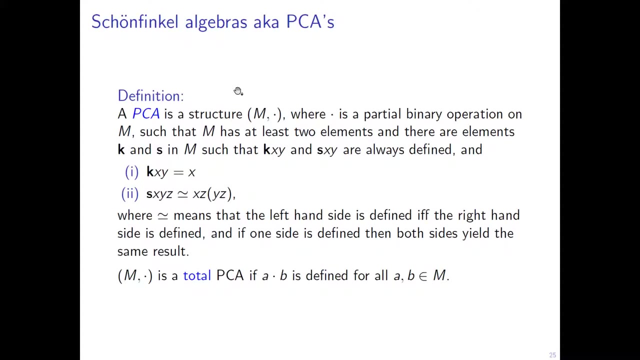 So then one does not need all of these operations, because F, C and S suffice. So this is the notion of a partial combinatorial algebra. Schoen-Finkl also did that. Okay, so the Schoen-Finkl algebra. 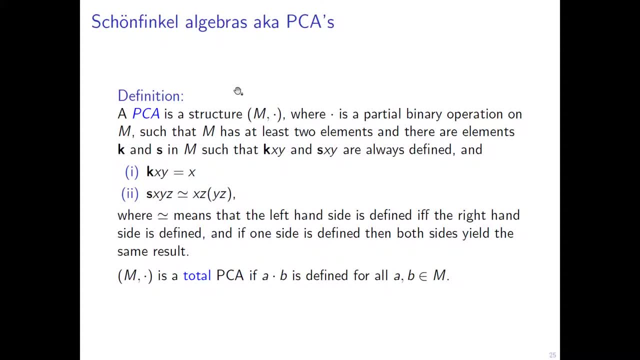 or partial combinatorial algebra. that's a structure where we have some kind of partial operation dot here And then one leaves out the dots. so K X, Y means yeah, it means K, dot, X, and then parentheses dot Y. 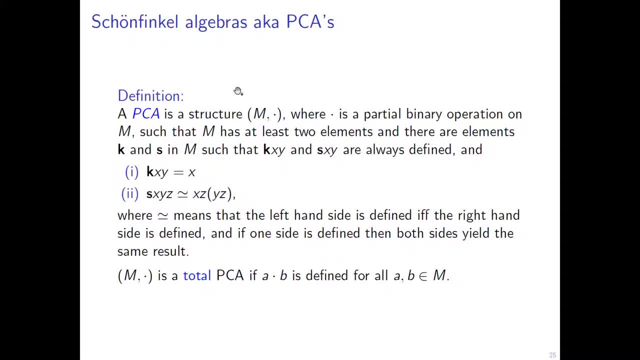 so it's bracketed to the left And then one just has these basic laws about K and S for Schmelzl, and that's this simple structure That's called the PCA, or Schoen-Finkl algebra as Peter Johnson calls it. 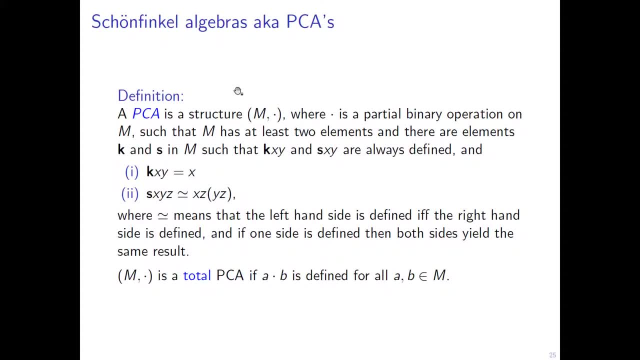 And okay, And usually to point out that this is a partial operation, so you may want to apply some object of M to another object of M and there might not be an output. But there are also PCAs which are total in the sense that there's always. so if you apply A to B, then you always get. 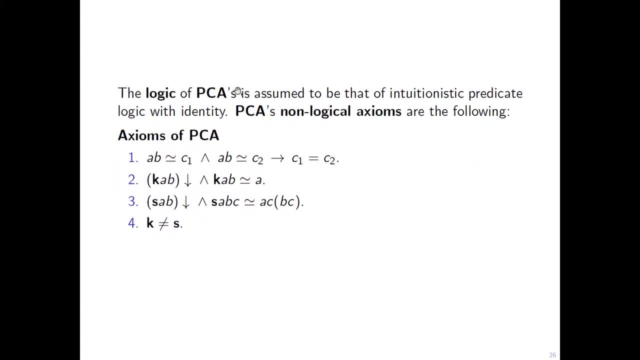 a result. Those are the total PCAs, And so you can make a theory out of it. let's call it PCA- I think that's how Beeson calls it in his book- with these basic axioms here, And you can also beef up these structures And then they have different names, I think. 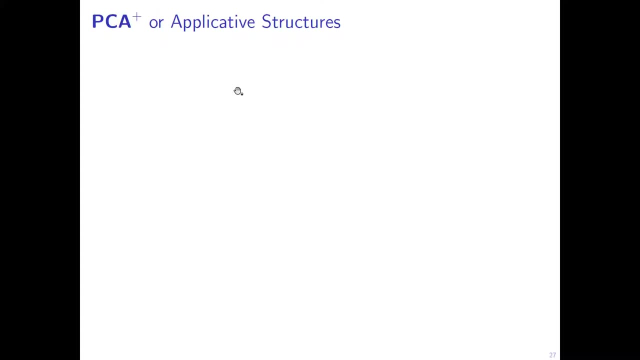 Beeson calls them PCA+ and others call them applicative structures. So in addition to the combinators K and S, what they do, you can actually now define over such a structure. you can define a pairing operation To get all the projections And you can define a certain copy of the natural numbers. That's 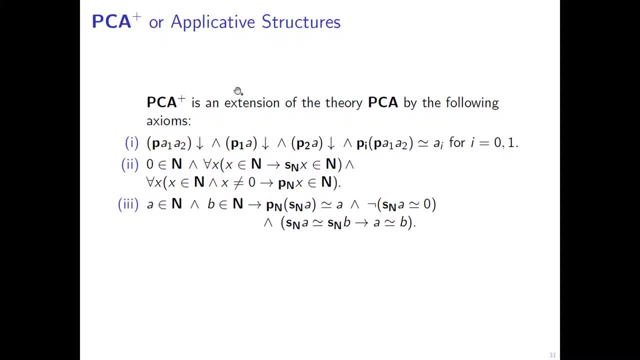 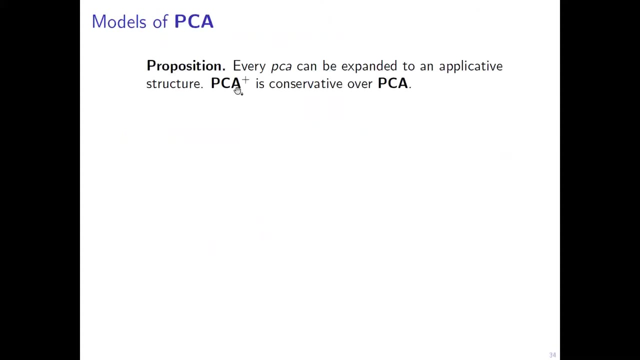 not so important. But what is important is that you can also define some kind of case distinction over this copy of the natural number. So this is important if you want to do realizability, this D here. So, but it turns out that it is already enough to have a PCA, because you can always beef. 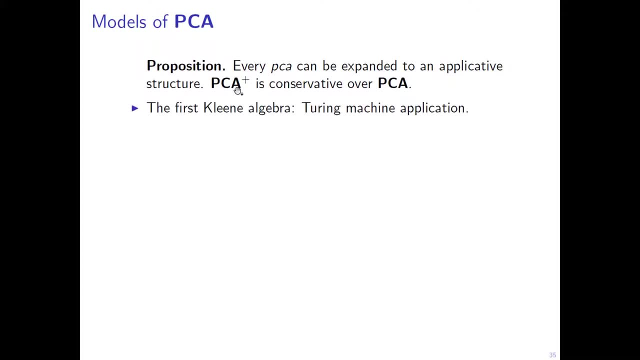 it up To a PCA+, Okay. And this notion has many, many, many applications, many examples. So we saw already the first, cleaning algebra, so Turing machine application. Then there's the second one. So here the underlying space is bare space, and then you do continuous function applications. 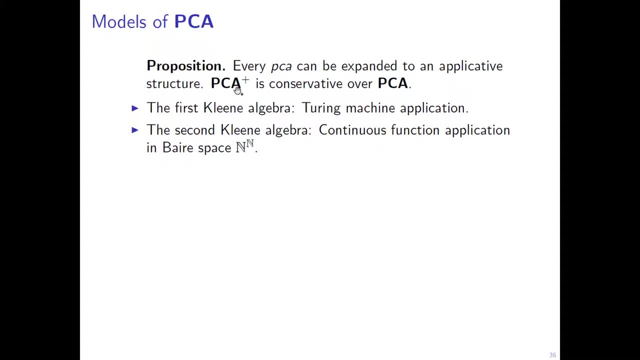 So, basically, you apply a function to another function by looking at the, basically the initial segments of the of the second function, until you get a result that is bigger than one, bigger than zero. That's the idea, And okay, Term models. 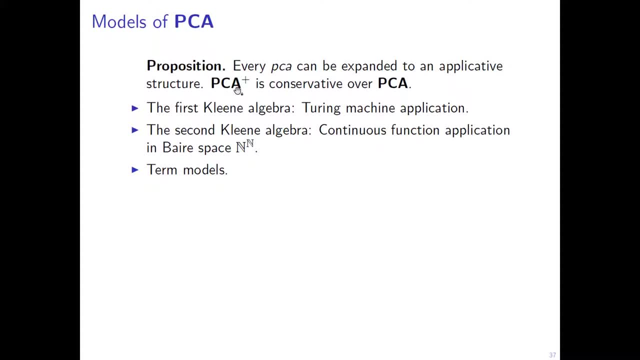 you can also out of syntactic stuff you can build wonderful PCAs. There are these more topological PCAs that also total the number of functions, And then you can also add sub-structures but also total. like what is the graph model, add its sub-structures. 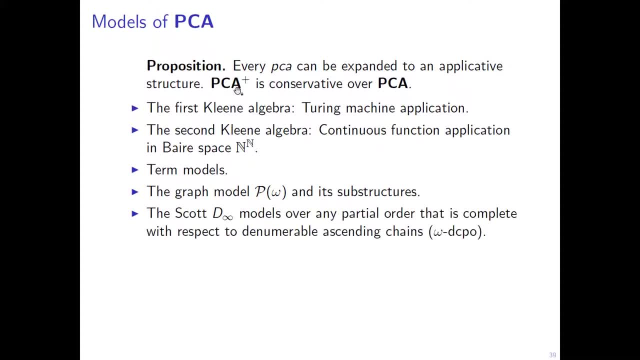 Then D infinity. it's got D infinity models. That is interesting because it's also extensional And there's lots of other examples. Non-started average, non-started model of the egg is rise to a PCA. You can do recursion over sets, admissible sets, higher type function nodes. 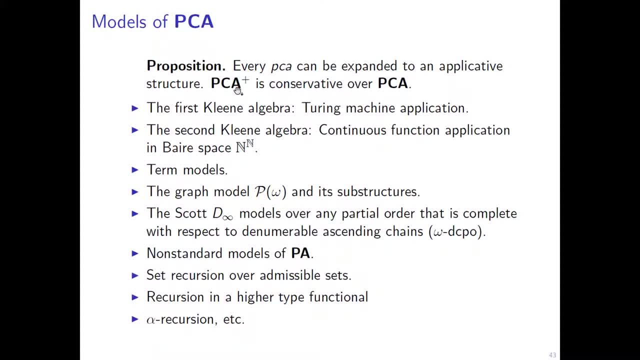 alpha-reduced, alpha-reduced. So you can do recursion over sets, admissible sets, higher type function nodes, alpha-reduced, alpha-reduced, et cetera, et cetera. So it's a very rich notion You can also look at. 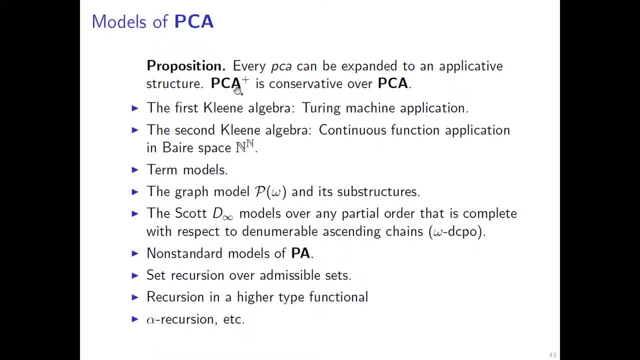 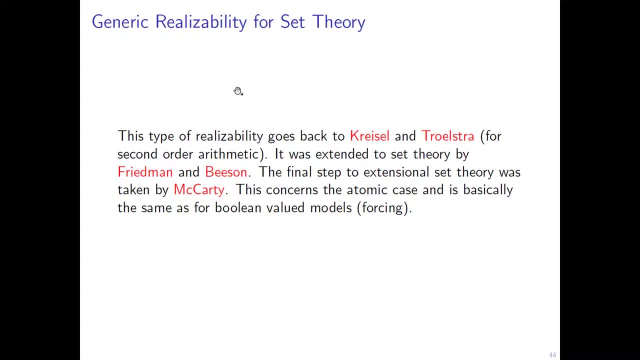 PCAs that are actually large, like classes, and then look what happens. Okay, Right, So for so this business of showing that intuitionistic systems enjoy certain derived rules, like the numerical existence property. There's a number of different ways to do this. There's 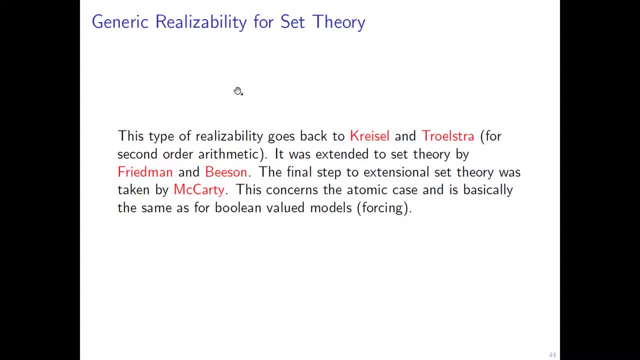 a notion of realizability for set theory, which is very useful. The roots of this notion go back to Kriesel and Trolster, when they wanted to extend realizability to second-order arithmetic, to intuitionistic second-order arithmetic, And then this was extended by 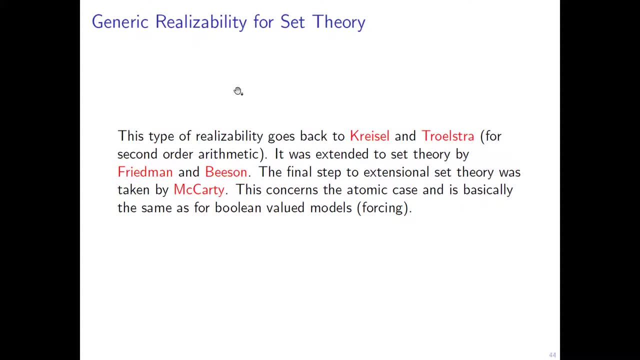 Friedman and Wiese to set theory, and though Wiese mostly used intentional set theory- without extensionality, I assume- And then McKernan showed that doing a set theory is possible. What we're trying to do now is the three-dimensional set theory. So you can see the set theory and want to get the set into your set theory Now, so I'll talk about ways we could actually do that. So let's go back and look at the method of mutation. There are a number of methods that can be used. The one that you see was actually the second-order method. I'll keep 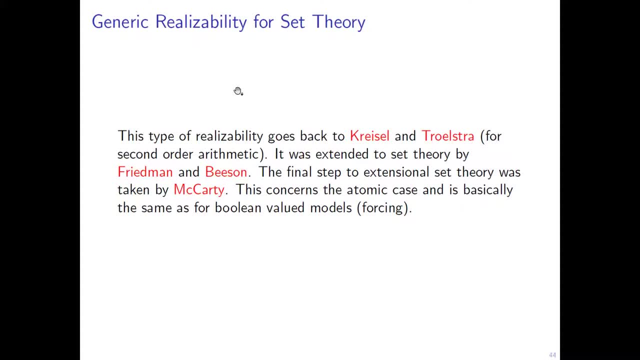 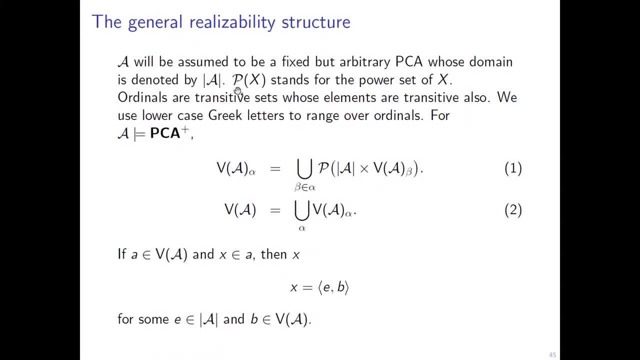 did the final step to extend it to an extension of set theories. Okay, so I don't know how to go through any technical details in there and mostly just skip these definitions. Okay, so the thing is here that realisability is not directly done for the sets of the universe. 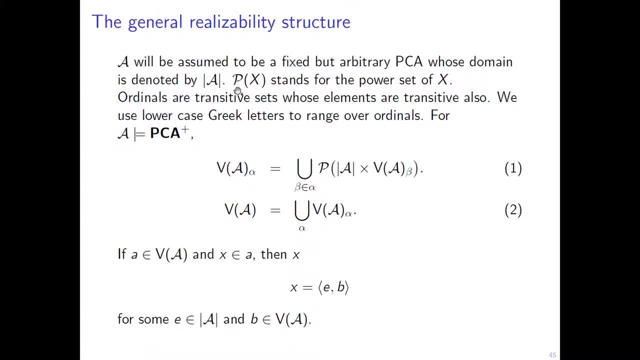 the set universe, but you first create a realisability universe, And this is the definition here. So it's some kind of phenomenon hierarchy where the given PCA plays a role. It's based on this PCA here, And so what you do is basically what you do is if you want to create this here. 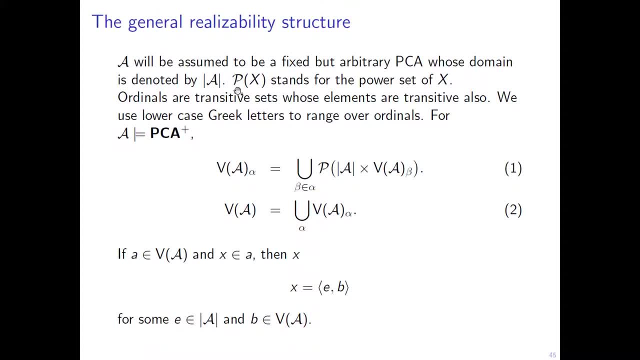 the alpha's level of this hierarchy. you take the power set over the set, Or the partial-corrector. algebra A cross the previous levels. So what it means is that if you now look at an arbitrary, so if you take the union of all of these levels, that's your realisability universe. 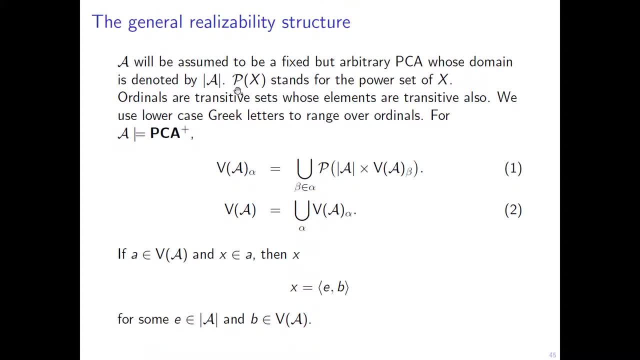 And then, okay, if you now look at an object living in this realisability universe, A well, how will it look like? Well, it will be a set, yeah, And the important thing is if it has an element, if there are elements. 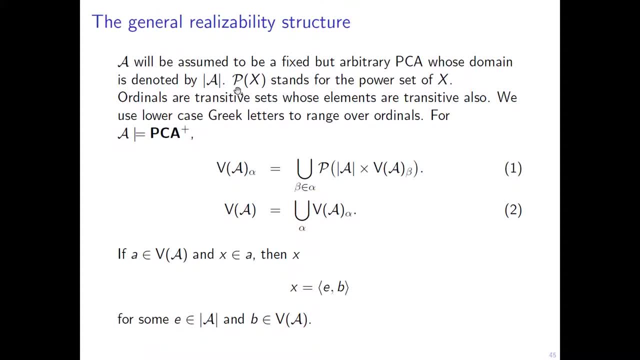 X and Y and A, then they look like this: They're always pairs where the first component comes from the partial-corrector algebra A and the second, B, is again a denizen of this universe. V of A. 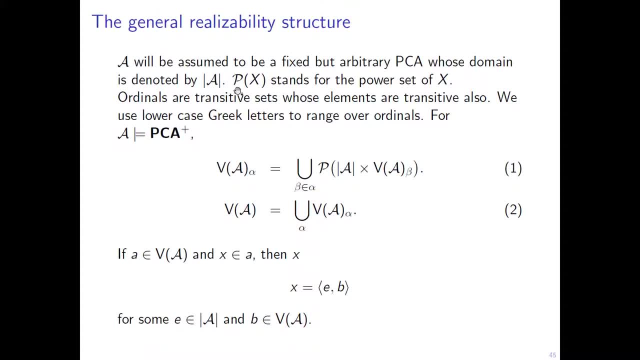 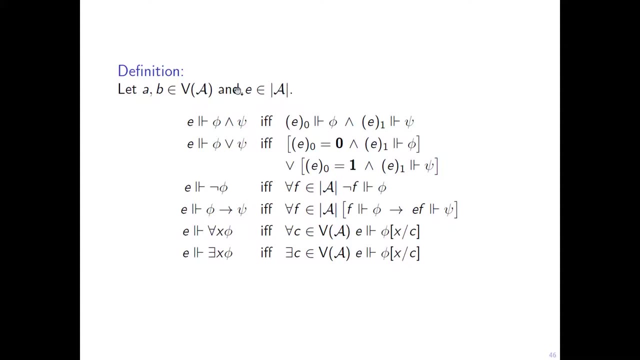 So you see, what now can happen is that the elements of the PCA, they can now act somehow on the first component of these elements. Okay, And then okay. then this gives rise to a realisability notion, and I just want to point out one thing. 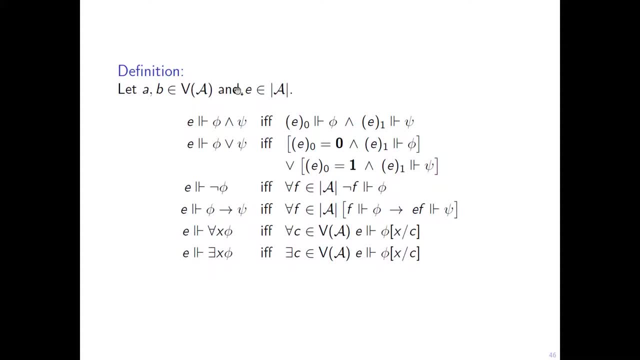 So here, this is peculiar about this notion of realisability is that a realiser, so E realises a universally quantified statement and it basically just marches through behind the universal quantifier. It just means that for all C in the realisability universe, E 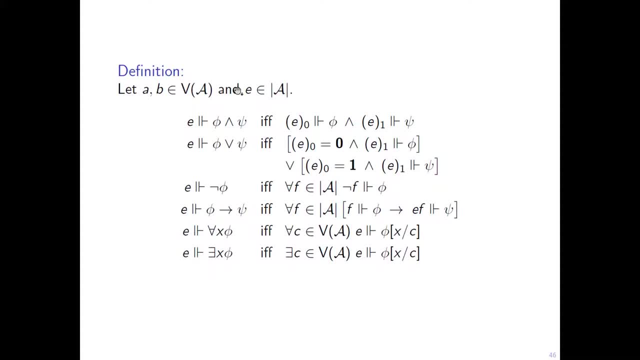 realises the statement here, phi C. So there's one reason why it's always the same reason. so it's kind of a generic interpretation of the meaning of truth in this universe. and the same with the existential quantifier. Okay, the atomic case is a little bit involved, it's clear. 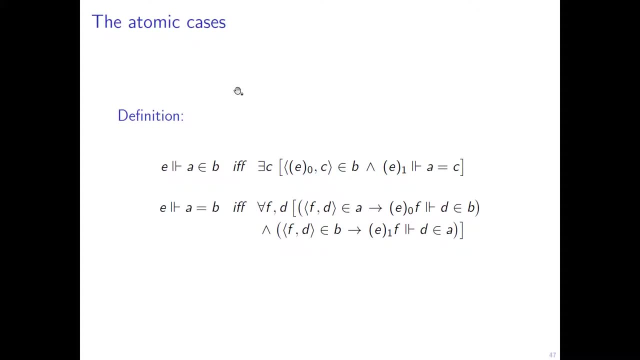 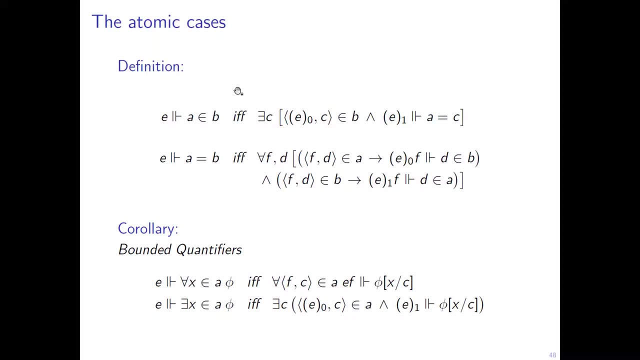 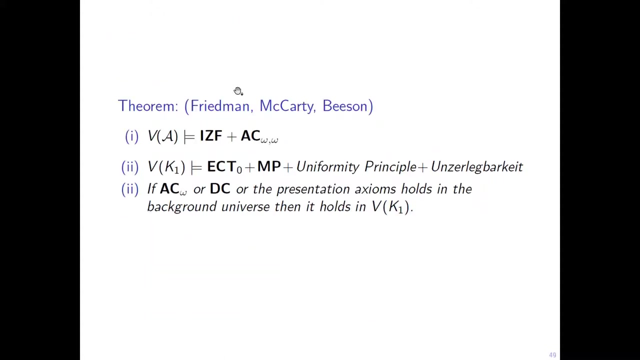 because it's yeah, it has to go by the build-up of these objects. It's similar to how you do it in four-speed And yeah And right. So I don't want to go into these details. So what happens now is with such a notion of realisability. 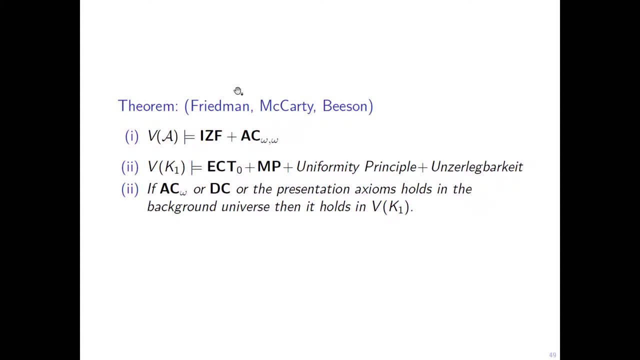 you can show lots of things You can show. it's a model of IZF that satisfies the particular form of the axiom of choice but not general choice. And if and then if you specify the, the partial combinatorial algebra, here to the K1, the first linear algebra. 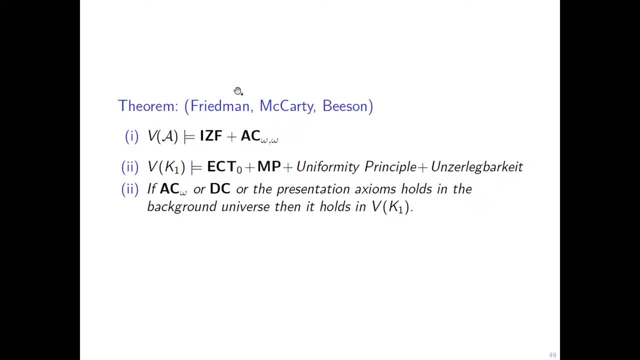 then this will be a model of the extended Church's thesis, of Markov's principle, the uniformity principle and many other things. And also if, if your background universe satisfies certain forms of the axiom of choice, like counter-choice or DC or the presentation axiom. 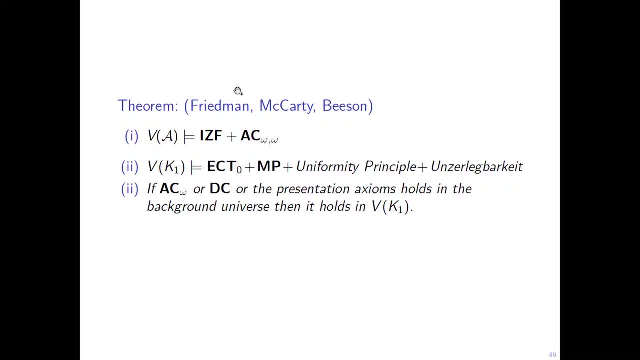 then these axioms will also develop, develop in the realisability universe. Okay, And now? basically, you can also view this as a way of explaining certain forms of constructivism. So this, the first, gives you Russian constructivism and the second Brauer's intuitionism. 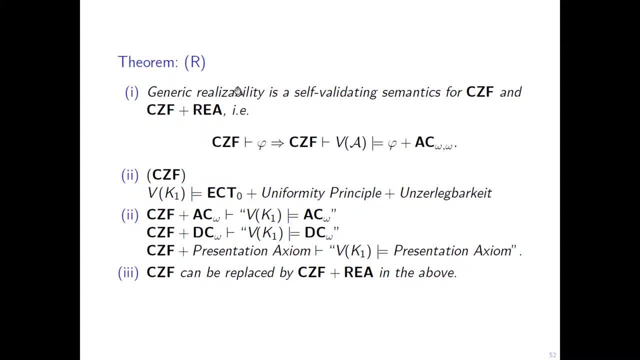 Okay, Just one remark. So the whole thing. so it was done for IZF, but it also works for constructive CZF And the important part is that it's kind of it can be internalized, So it's it's self, it's a self-validating semantics for CZF. 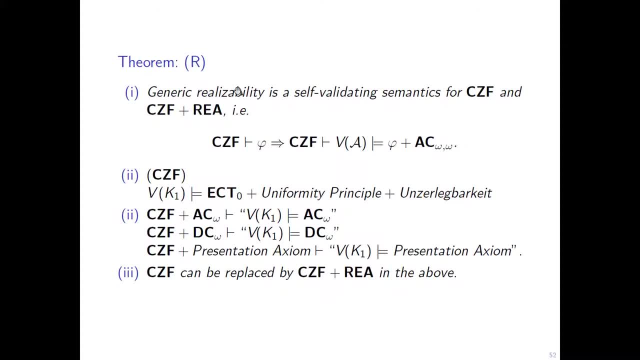 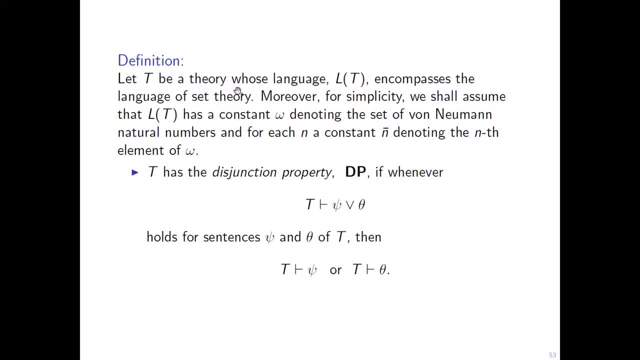 and several extensions of CZF. Okay, So now some of these derived rules that many of the indigenistic systems have, so the disjunction property. so if you prove a disjunction, then the theory proves one of the disjuncts. 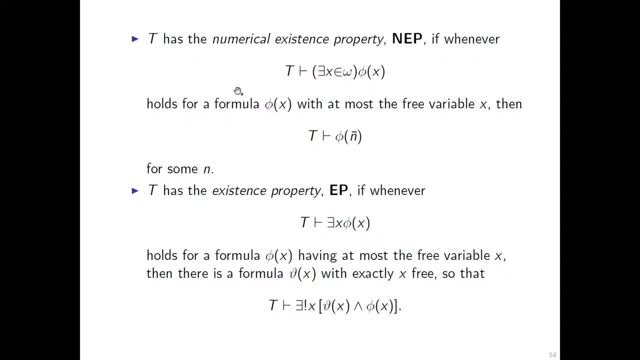 And the numerical existence property. now, since we're working in set theory, we have to. so it means if we prove an existential statement that some number exists, an omega 5x- then one can find a numeral n so that t proves phi of n. 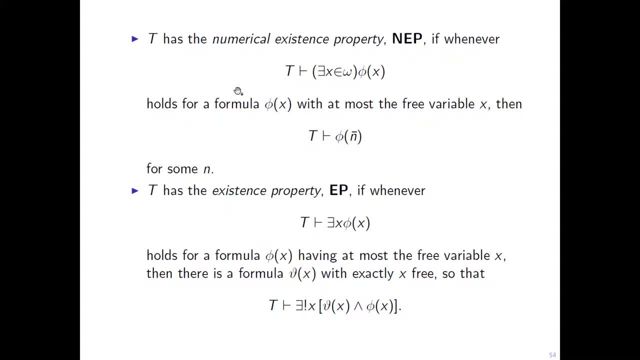 So it's a question: what? do we have these terms in our language or not? Well, it doesn't really matter very much. So either this: either you have these terms in your set theoretic language, you just add them, or you. 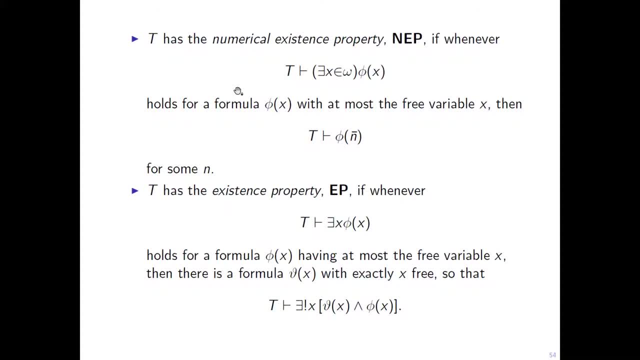 or it means you have. you have a certain description of this n here in a certain simple way. Anyway, there's also the existence property, where there is no restriction as to where you find these objects, or this is an existential quantifier over the entire set theoretic universe. 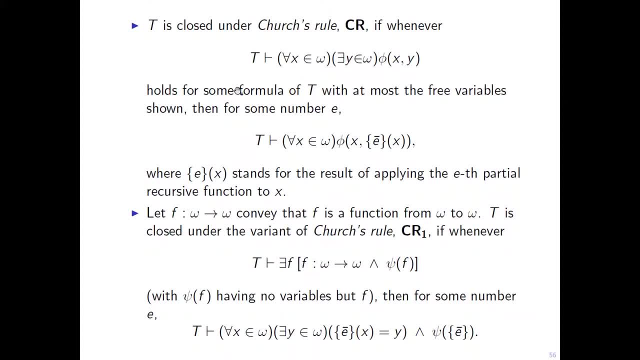 Okay, and then lots of. there are lots of other things like Church's rule means: if you prove a combination of for all x and omega- there's a y and omega of phi xy- then this is witnessed basically by a. 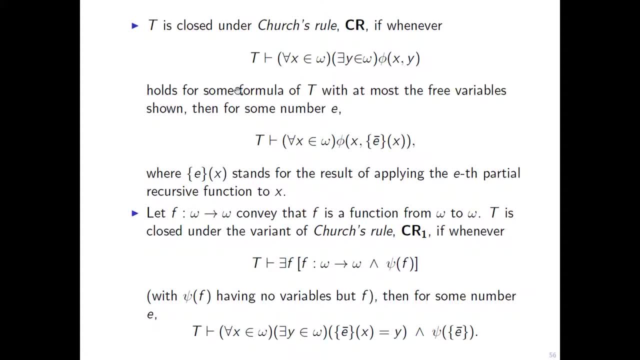 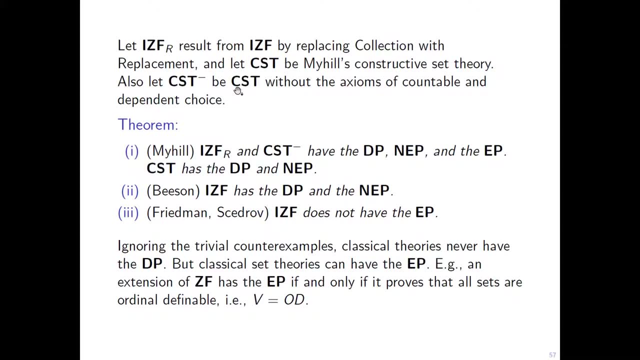 by a computable function. So that's the Church's rule, and there are many variants of it. and then it turns out that, yeah, many of these intuitionistic set theories have these properties, For instance. so Meyer proved it for his. 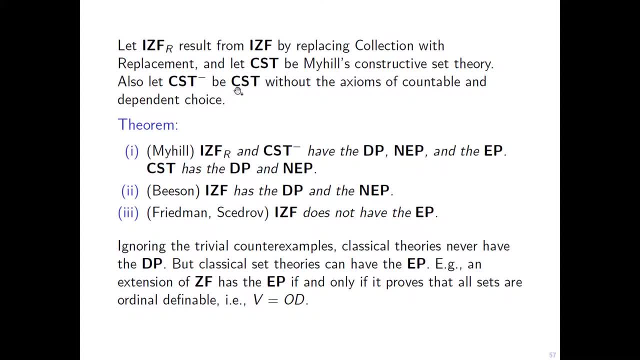 for IZF based on replacement, and for his CST, Beeson proved it for IZF. IZF is usually based on replacement, IZF is usually based on collection, not on replacement, and so on, And so these systems have the numeric existence property. 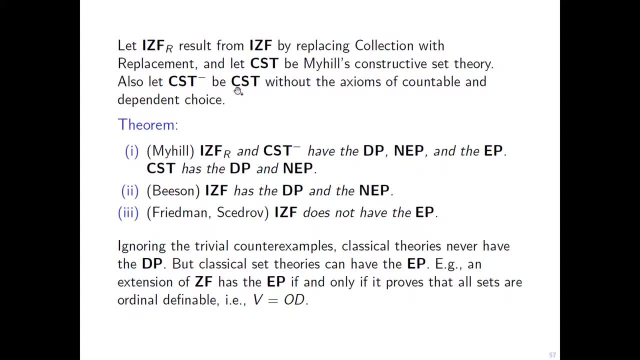 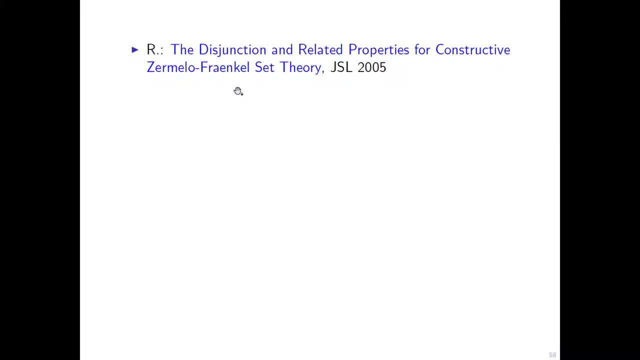 for instance, An interesting case is that IZF does not have the existence property And but I don't want to talk about this. So the methods that they use are different and they usually, many of the proofs- go through some kind of intentional set theory. 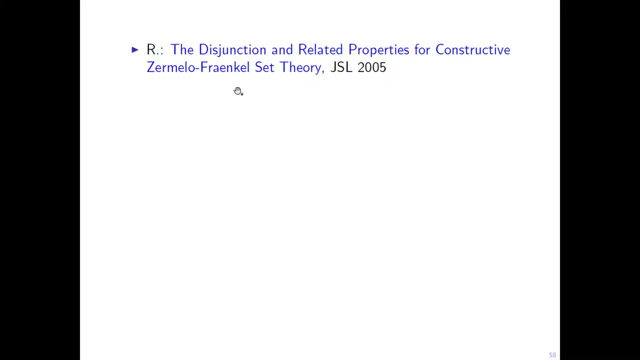 and then have to go through and then have to say something about how intentional set theory can model extensional set theory. Okay, so I was interested- this is looking back in general machinery- that this would work for almost all of these set theories. 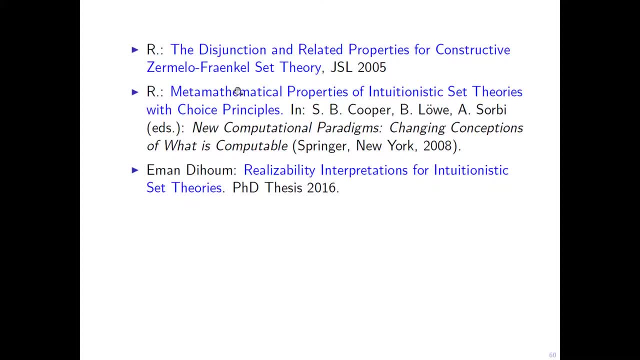 and the idea is that there should, so there should be a general machinery, and the rough idea was that, okay, we have this generic realisability. what we have to combine is truth. So this realisability is truth, And so this was in. 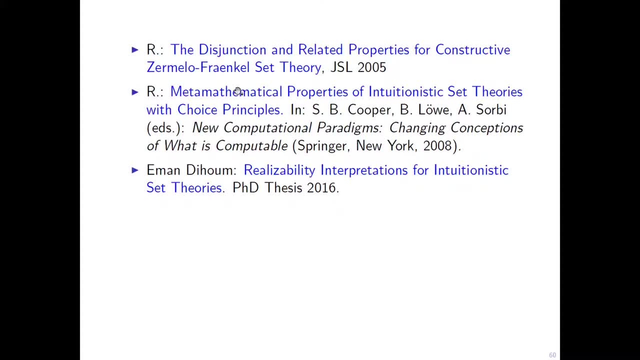 yeah, in the early 2000s, but recently it was- this kind of topic was taken up in a PhD thesis by Iman Dihoun. so she- yeah, she received her thesis in 2016.. Okay, and so the problem is now that, at the same time, 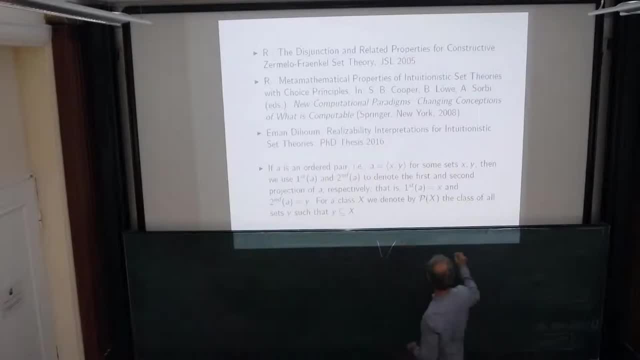 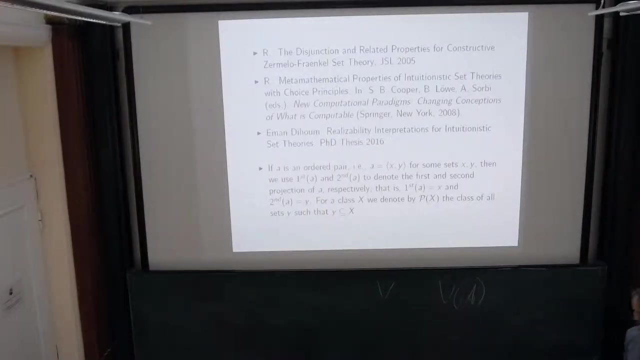 we have to talk about the universe and about the realisability universe at the same time, And so what we would like to have is some kind of realisability that talks about them simultaneously, And the rough idea is that this new realisability universe 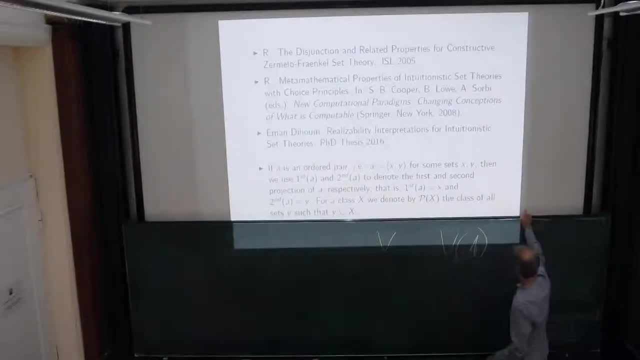 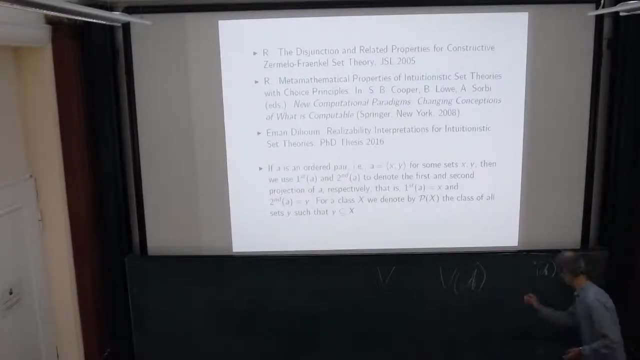 which kind of combines the two. let's call it V star of A. the objects in this universe are pairs of objects, AB. so this is X and in a certain sense it's a. it means that this, the first component. 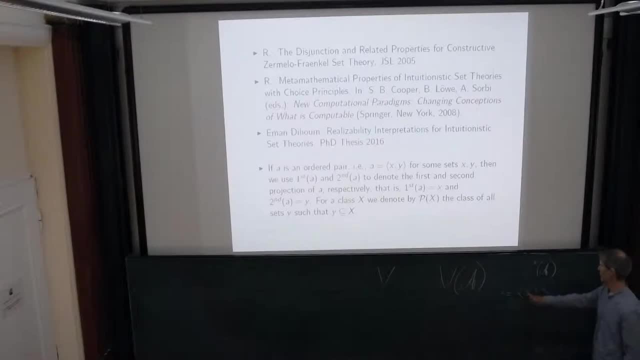 the first projection is considered to be the real part. the first component lives in V and the second component lives in V, star of A. And of course you don't, you cannot throw together two arbitrary things. they have to interact in the right way. 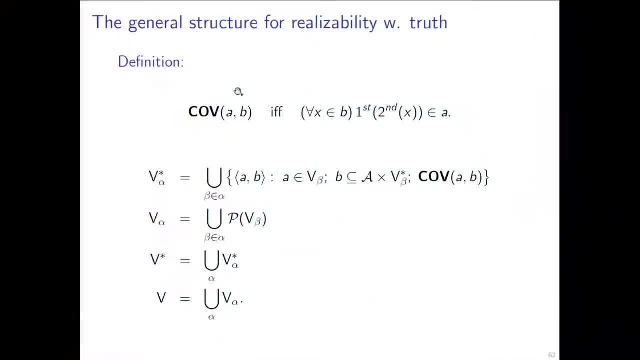 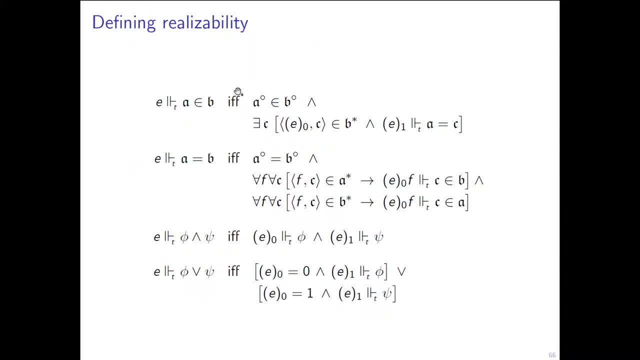 and that makes it a bit involved And I do not want to go through these details. Anyway, there's a notion of realisability with truth and um and that um. okay, that's here are some of the clauses. 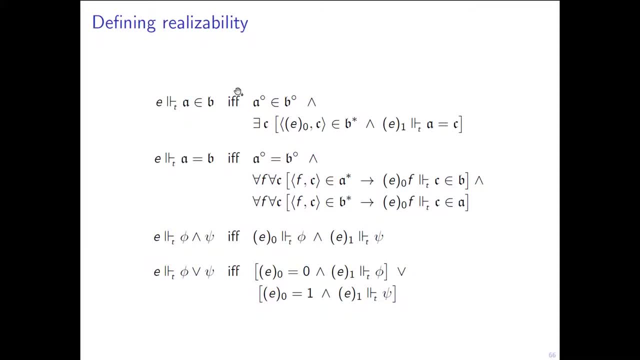 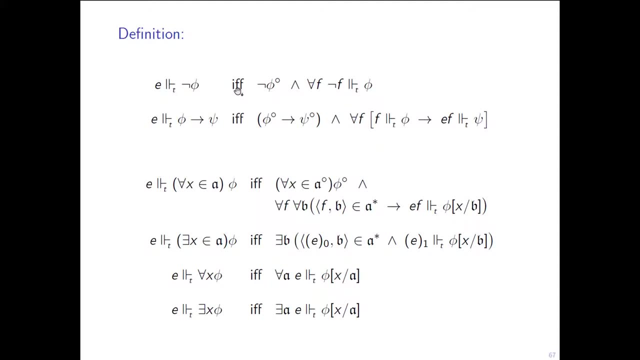 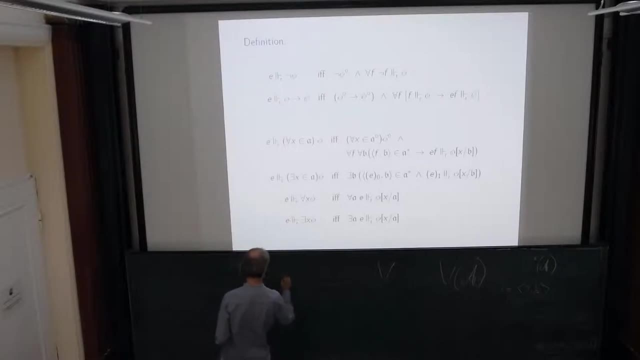 So I just would like to point out where truth plays a role. Um, if you have a statement now a statement, say um phi, and these AM live in, these AM are um, these objects from V star A. 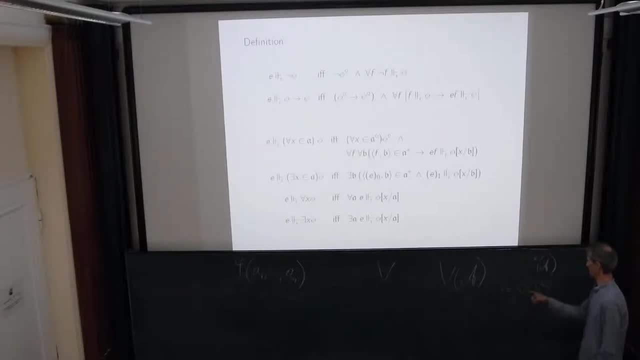 yeah, and, and those objects are pairs and so the first component therefore lives in V, And so if you do the following, if you take the first component- yeah, this is this operation, uh phi with an. 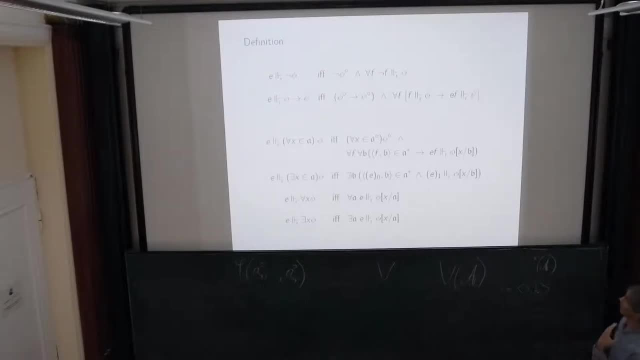 with an O as a superscript. So every statement that you have about the realisability universe has a counterpart in the background universe. yeah, And so to get to this truth, uh, just let let's look at the implication case. 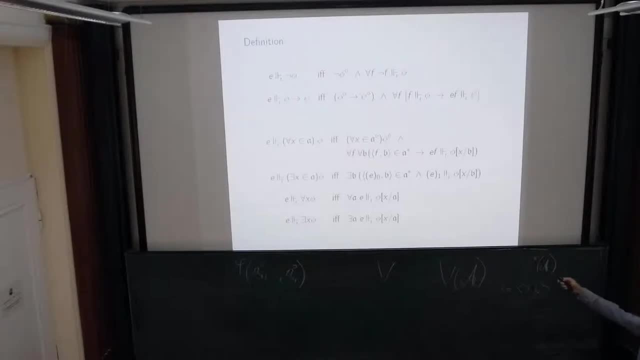 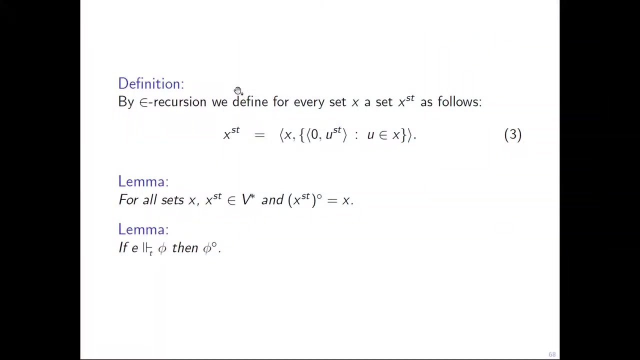 So here is: this is the usual realisability software implication. but then you also require that the implication is true if you look at the real parts in the real universe. Okay, Anyway, so this whole thing works and in the end, 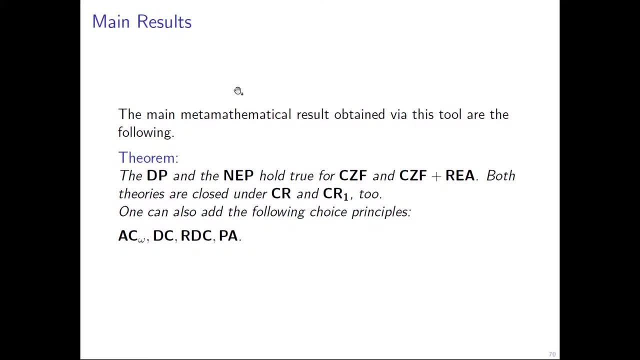 um, you get from this machinery, you get that, uh, all kinds of set theories, intrinsic set theories, uh, satisfy the numerical existence property. So I mean here I just mentioned CZF and CZF plus real. This is a theory where you can do inductive definitions. 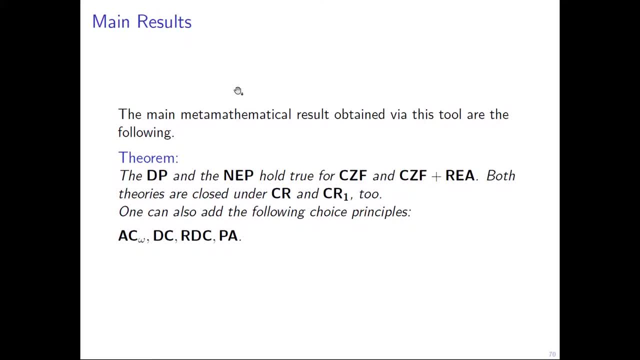 but one could uh take IZF real. One could also take IZF with large uh set axioms, like uh measurable or whatever, and it would still work. It's, it's. it's a very general machinery. 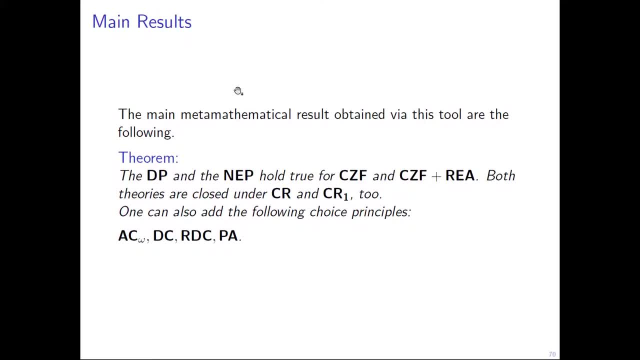 It's very robust. And also you can add, uh, choice principles, uh, that are, um, not in contradiction with intuitionism. So the, the cultural action of axiom of choice, dependent choice, and so PA. 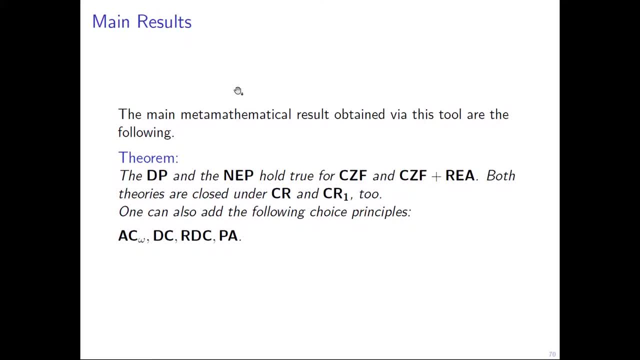 here stands for the presentation axiom, not for Okay, Right, And and so you, you get all these. um, it's, it's very general. I thought that, um, that's a very general example. It might be useful. 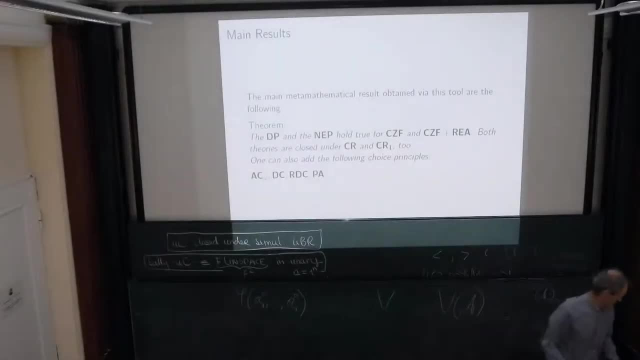 So, for instance, um uh, the numerical existence property also is uh interesting from the point of view of type theory, where it's sometimes called the, so that if you have uh in particular with the connection with um. 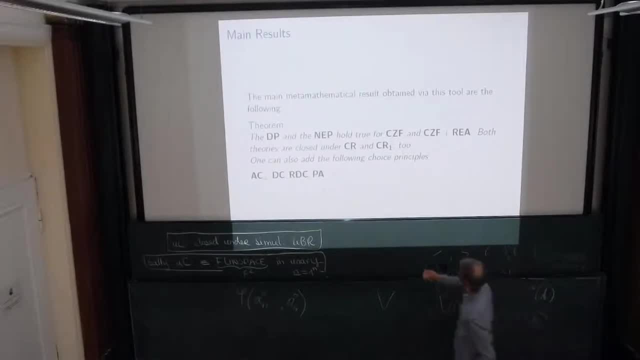 homotopy type theory and the. And the thing is that between type theories- Uh, although very often it is explained that the, that the set theory is totally different from the type theory, but there are connections you can interpret back and forth between the two here. 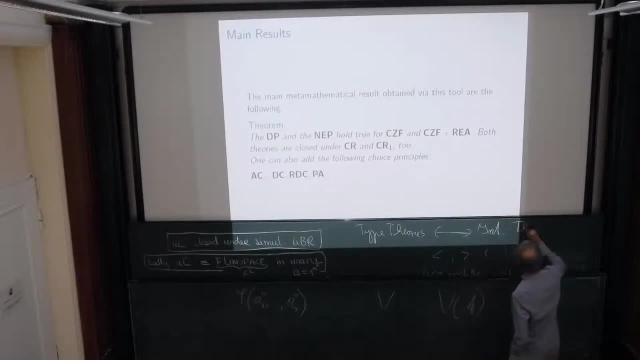 Yeah, So that's the interpretation that gave, but there there are also interpretations now that are that are somewhat informed by um, the um, by homotopy type theory, by the age levels and and and. 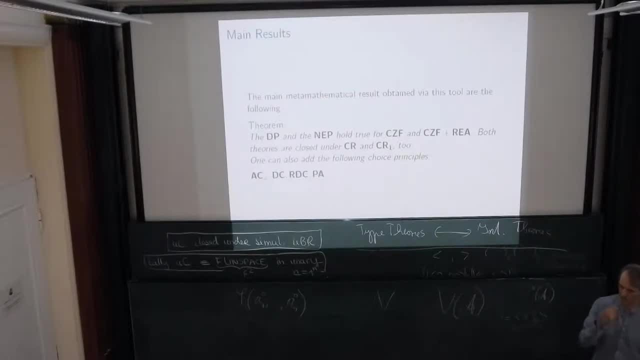 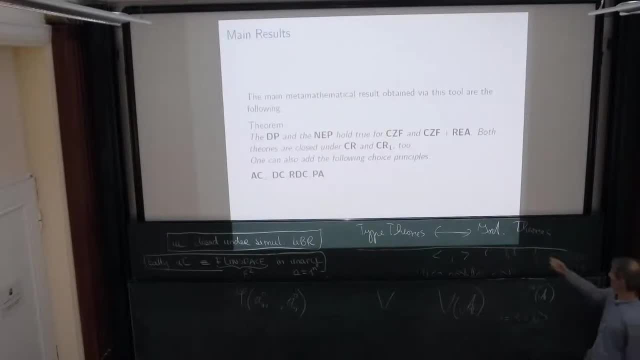 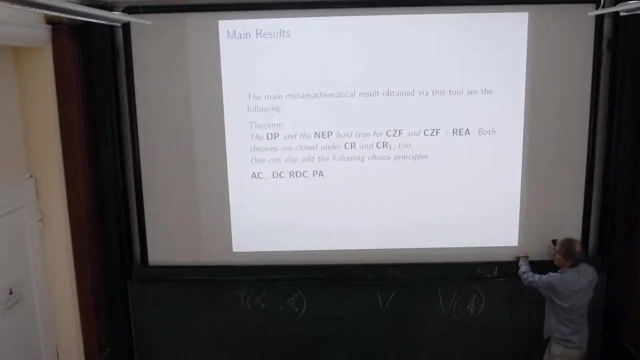 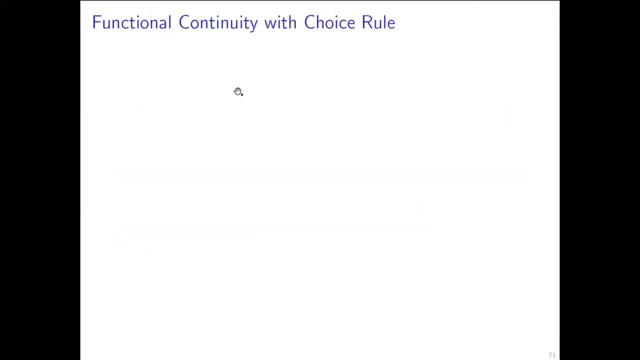 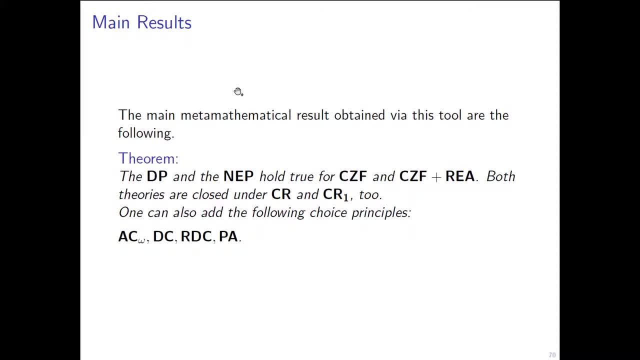 the paper just uses one PCA, mainly Kleene's first algebra. yeah, So now what about all the other ones that we have? Can they also be used? And, of course, an obvious question as well- What about the next, the Kleene's second algebra? 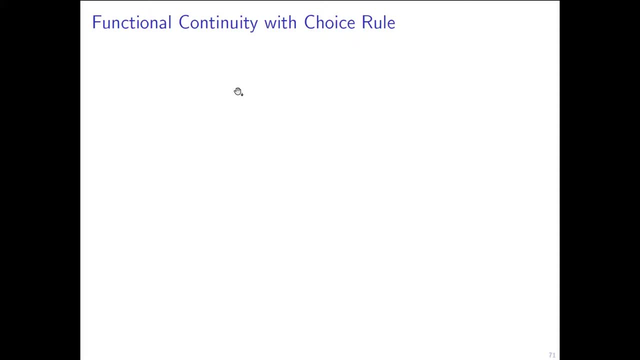 where we have a continuous function application And, yeah, it turns out. so there are also rules that are kind of germane to this, to Brauerian intuitionism, like this rule here of functional continuity is choice and many other principles yeah. 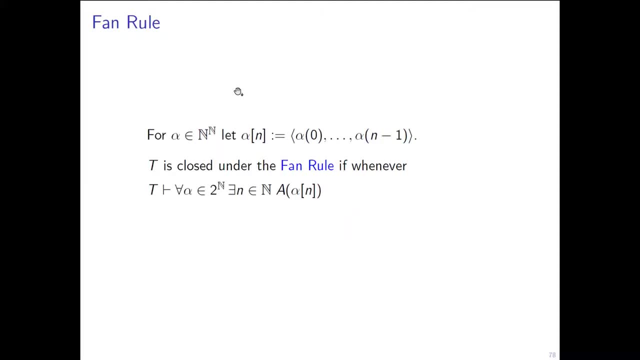 And the fan rule, for instance, and the monotone bar rule is the rule version of monotone bar induction, And it turns out that many intuitionistic centuries are also closed under these rules. so these are derived rules for those systems And, for instance, it has been investigated by Daniel Vandenberg and Michael Burdeik. 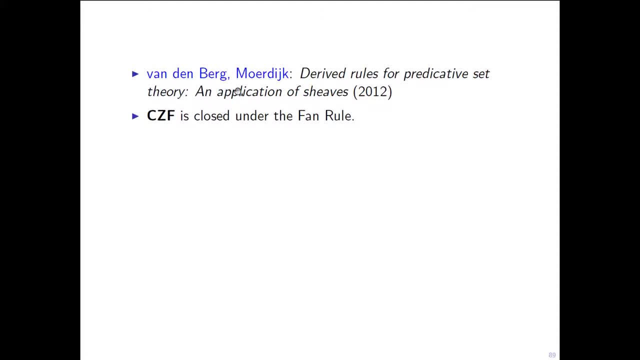 And with a very different technique, using sheaves For instance, they showed that this theory here, CZF with some additional stuff, is closed under the monotone bar rule. yeah, Okay, And it turns out that if you apply the 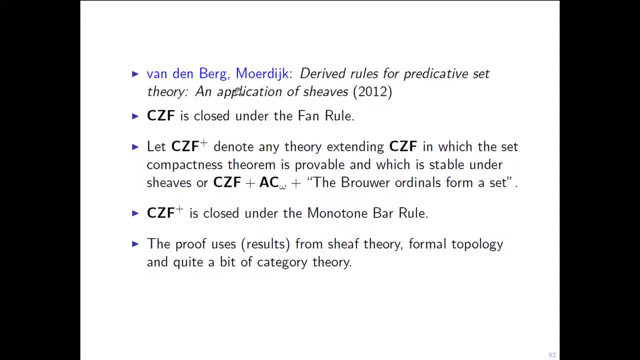 so this is, as I said, the techniques. so from sheave theory and formal topology, quite a bit of topology, pedigree theory one could also use realize GD's truth to approach these rules. And yeah, it turns out that you can also show this for CZF. 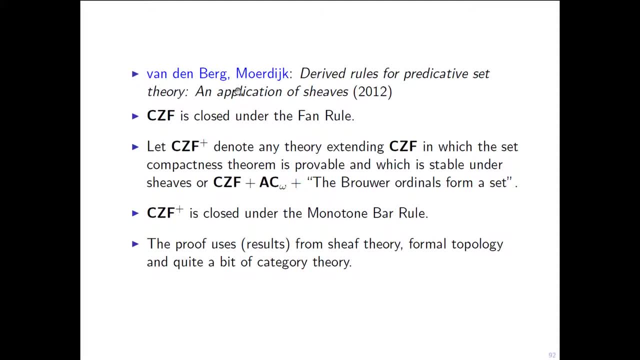 So this was for. so the closure under the monotone bar rule was for CZF+. So in other words, you have to have something, you have to have something more here, But this rule, also also CZF itself, is closed under this rule. 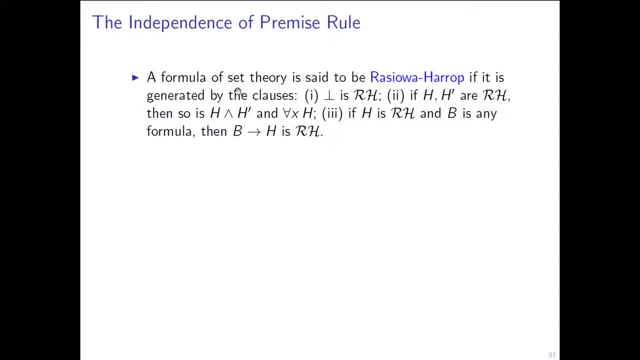 Okay, And many more. Just another example, because I'd like to finish soon. Another thing: another characteristic feature of linguistic systems is that they that they're often closed under the so-called independence of premise rule. That means basically that if you have a situation like this, 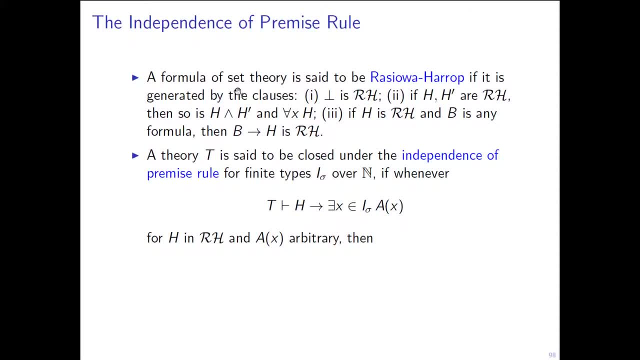 so T is again in logistic set theories And it's closed under the independence of premise. we'll say for finite types: I sigma If, whenever you can prove an implication, H implies there is an x and I sigma A x, where h has to be some kind of negative formula or Rassiola, Rassiola-Herald. well, 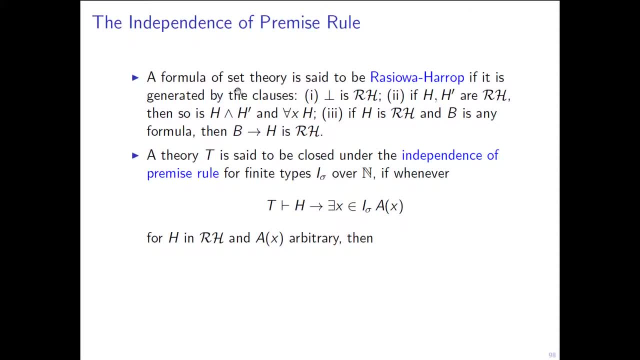 then you can pull the existential quantifier in front of the implication and yeah, so that you get something like this. Well, and it turns out that you can also use this machinery for such rules, to establish such rules, and one crucial feature here is: so, if you think about, say, Kleene's first, 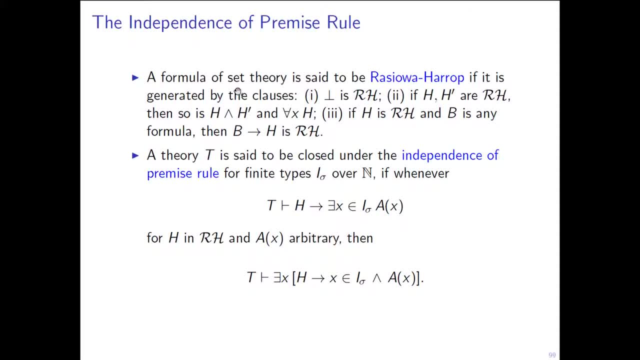 algebra or second algebra. they are partial combinatorial algebras and really, if you want to show this, the theory is closed under this kind of rule via a PCA. you really would like to have a total PCA. The reason is that 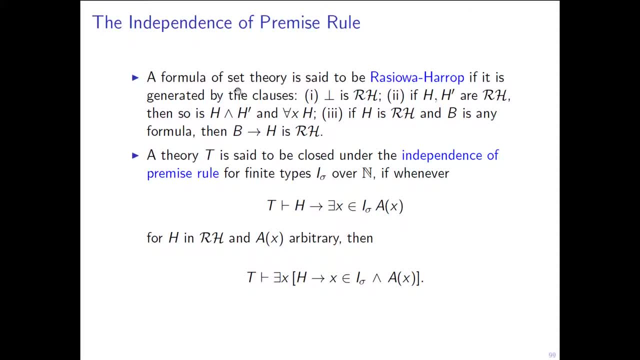 If you have a realizer for a statement like this, the h implies that right, so the realizer would act, would have to act on a realizer for h, where h is negative. so you know, if there is a realizer, then zero itself is a realizer. so then you would have, so then 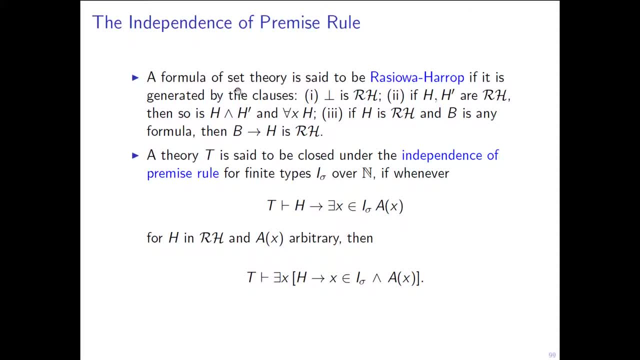 a realizer for this statement. say: e realizes h implies blah, so e would act on a realizer of, on a realizer zero for h. if h has a realizer, yeah. But what you'd like to do is you would like to apply e anyway to zero. then you can only 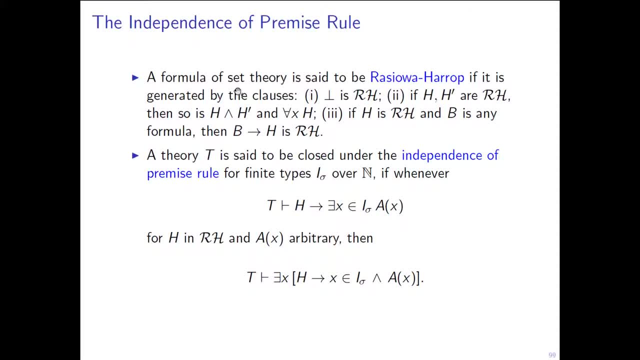 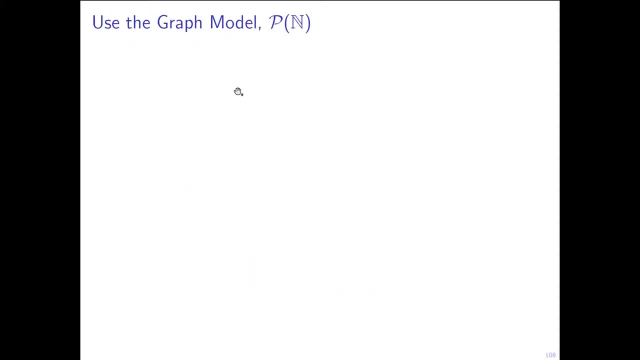 do. if you know it's total, yeah, So that's why totality comes in here, and then basically, this can be done, Okay, and so you can use, for instance, the graph model. this is a total PCA, you only. 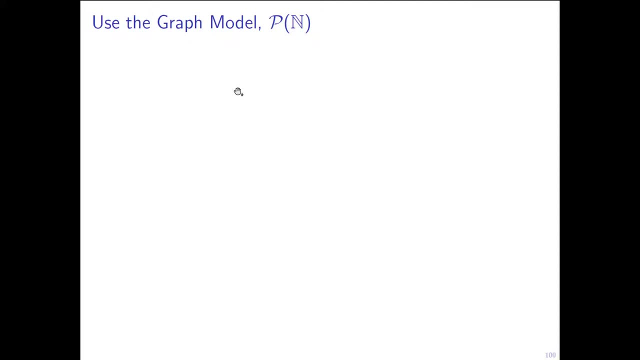 need a sub, a subgraph model. It's called complexity and anyway, so this can be done and so, yeah, there's some work with Takako going on, and I think yeah, and so if you have seen some of these football, 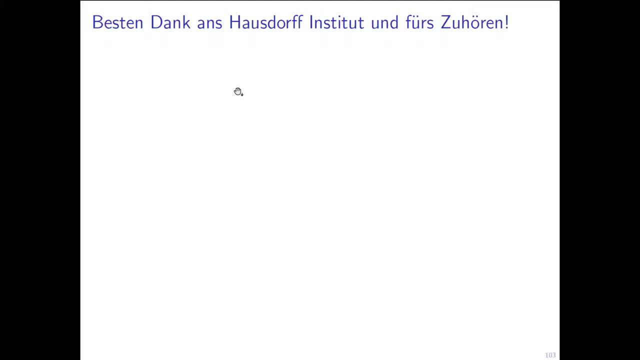 games, when the players are interviewed, very often what happens close to the mic? there are certain hotlines, like with Coca-Cola or with- I think in Germany it was, I don't know some beer. does anybody remember which beer it? 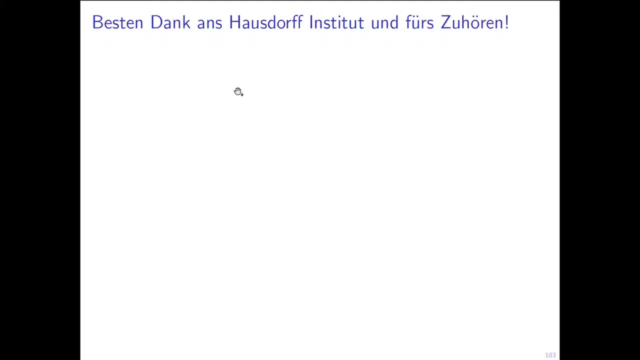 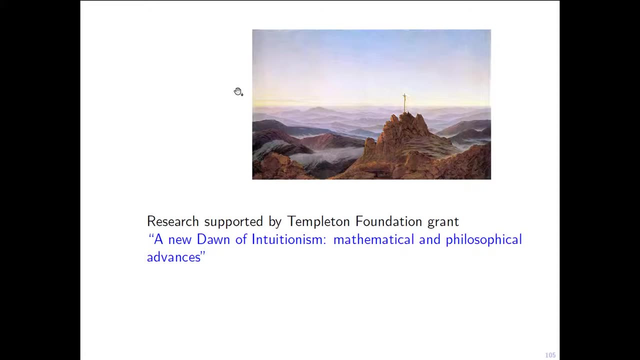 was. Was it Bitburger or something? Yeah, okay. anyway, I'd also like to say my sponsor. it's the Templeton Foundation, and so that's the end of it. Ah, I have forgotten something. Right, This is a cross we have on the table. 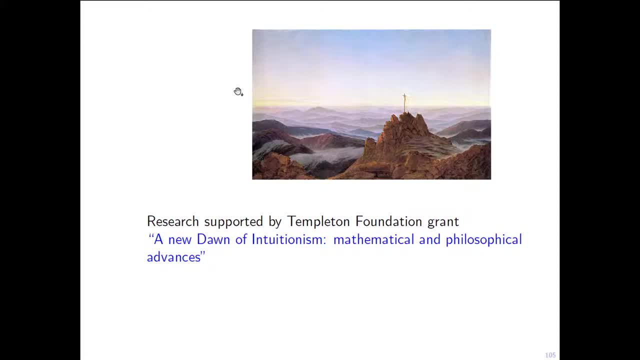 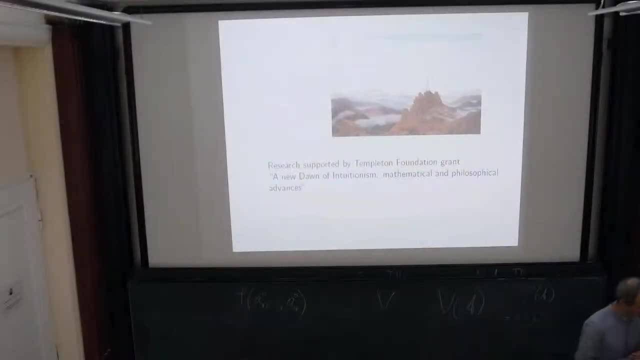 Yeah, I think I'm almost done. Yeah, I want to thank the organizers of this workshop and I think what my impression was actually that this kind of format of just 30-minute talks was quite nice. It was kind of refreshing and lively and I think it worked well. 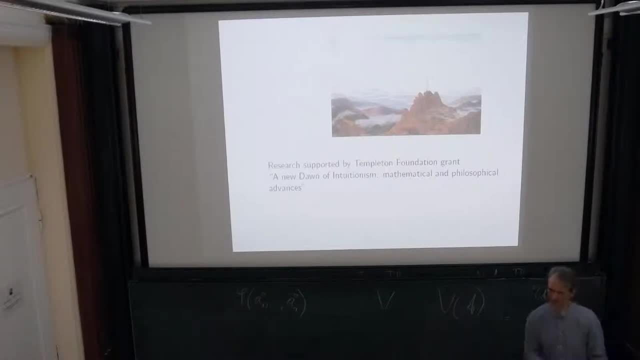 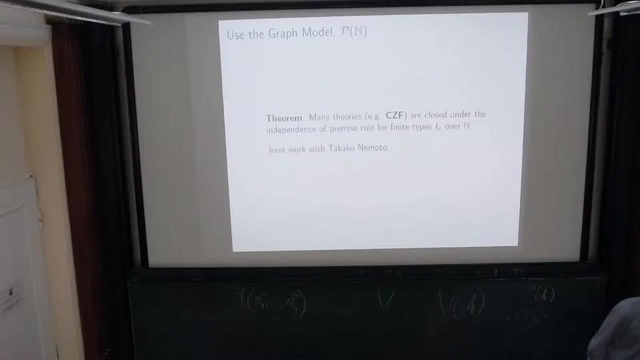 Okay, Whenever I see you, you've got to go back to the Okay, Okay, Okay interprets the intuitionistic version of Busser's theory T1-2, then for that interpretation it has the numerical existence, and if the theory has a disjunction property, 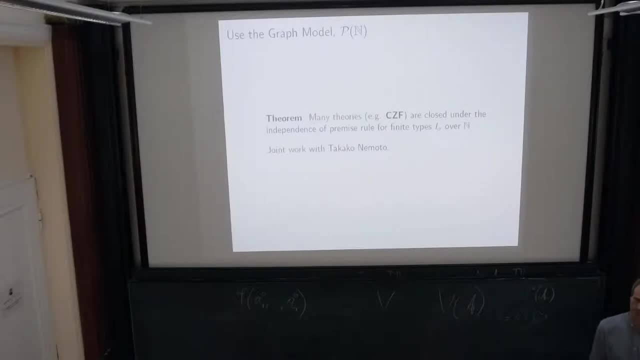 then it has a numerical existence property. so in all your examples the numerical existence property follows the fact from the disjunction property. yeah, that's right. very interestingly enough, there's a paper by Andrew Swan and myself where we look at other theories and in those theories, 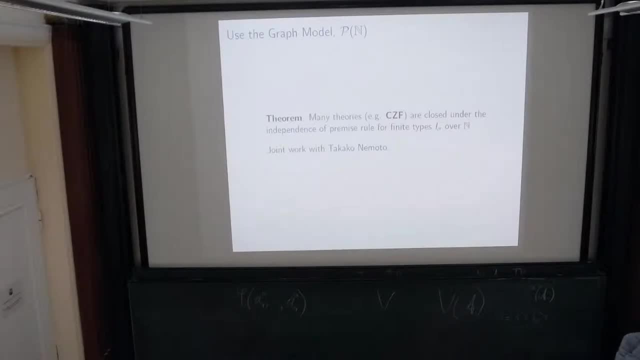 they do not have this equivalence. sometimes you can have the existence, the disjunction property, but not the existence property. but these theories are not recursively axiomatized. yeah, sometimes I just want to say that you can have one without the other. yeah, yeah, about this theory. finite types. 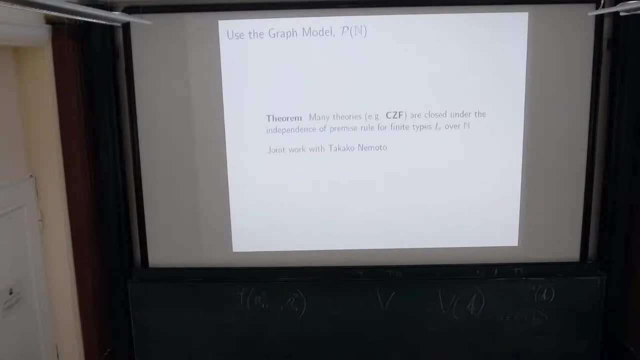 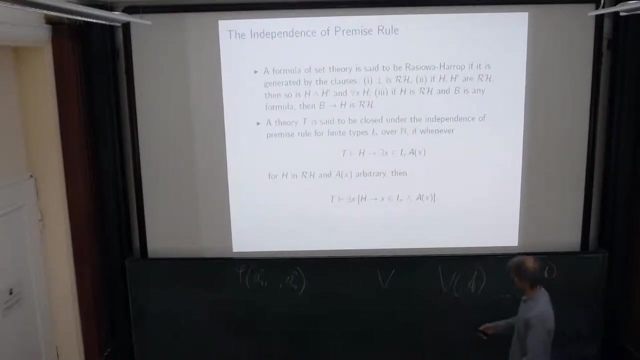 includes n finite types. yeah, finite types over the finite type. sorry, yeah, you basically look at solid. so that's, I think there's no hope doing this for an arbitrary set, right, so that you, um, you have to prove that there is an x and then you might think maybe we can put here some arbitrary set. 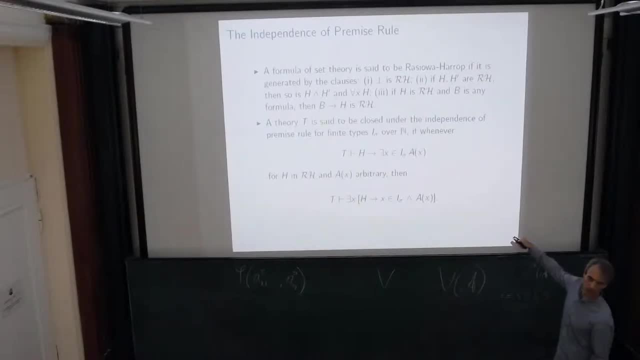 maybe there's a description, but then it usually wouldn't work. so it definitely works if you have. the usual case is that you look at the natural numbers here, right, so there's an x and omega and then you want to pull the x. is that the quantifier? 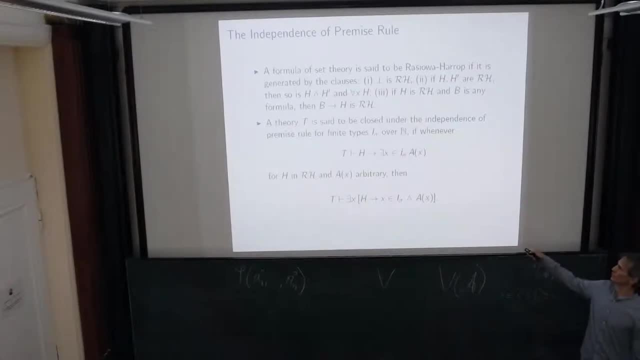 to the front. but then you can also do it if you, let's say, look at the finite types externally, built over over omega. yeah, so you can have bare space here and then higher bare spaces and so on. yeah, that thing is kind of so you have you use graph mode. 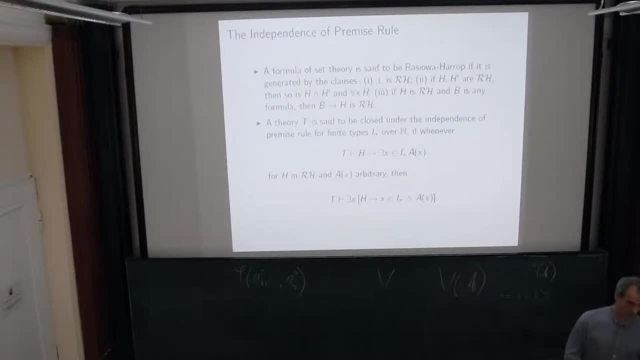 so omega is somehow interpreted as sigma. well, the graph, the graph model, is only used for the um when one builds the realizability model. so we stick in the graph model here. yeah, so in the case of heighten arithmetic and in the case that the h is a negation, 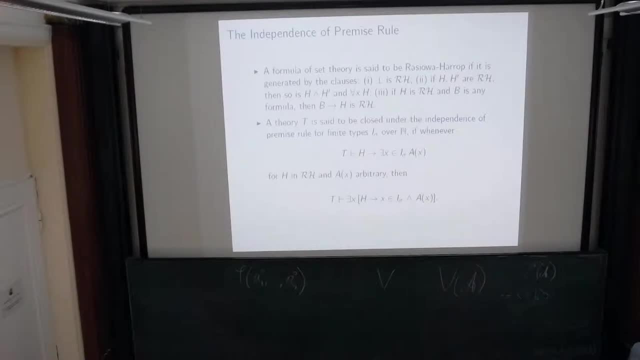 you can also do it using the friedman translation, that that way we lift it to the richer series. you mean this approach would work there? yeah, i don't know whether i could do it for the harold formulas in general, but if it's a negation. 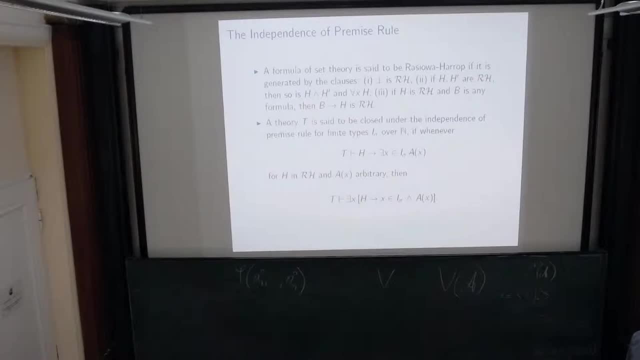 then the friedman translation would do the trick. yeah, it could be. yeah, i mean, um, there are. i guess i said there's a somewhere in the middle, but there are lots of methods for different methods, yeah, for showing, uh, for instance, the non-barrical existence property. 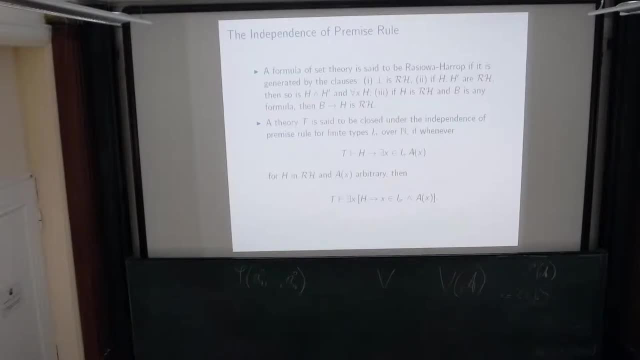 is system and, yeah, there might be another way. i think the idea, the idea is mainly that if you have a general framework- yeah, you have the framework already at hand- and then if you have a problem showing you want to establish some kind of derived rule, then you have to choose the appropriate pca. 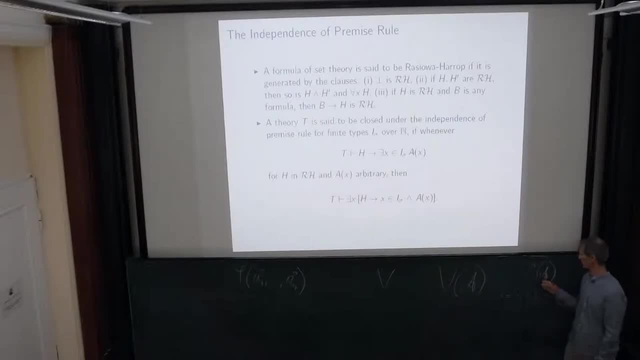 so it's nice to have a general machinery there, so we only need to specify this part. yet another question: so the um the series do not, uh, verify their own disjunction property, but there's a they cannot. they cannot, they're inconsistent, right, yeah? so on the punishment of proving their own inconsistency, 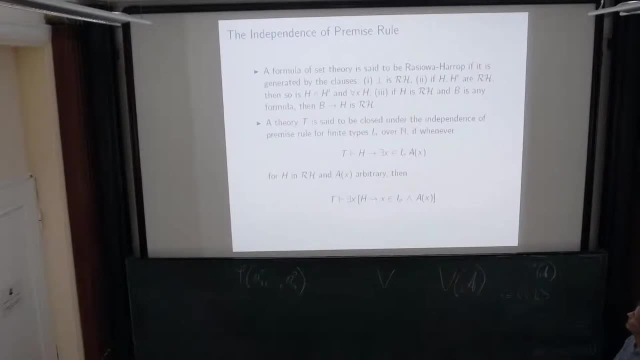 but there is a, an approximate disjunction, property that could be proved, and that's called the advanced principle, and it says that if provable a or b, then provable a or provable b. right, so you can. if you can prove a disjunction, you can. 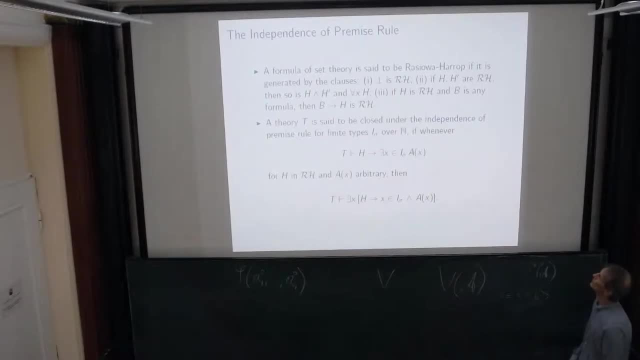 add a, a provability, in front of one of the disjuncts. so that's the advanced principle. and oh for h a. you proved that using q-realizability. yeah, so the the question is: can? can we lift lefant's principle to these, these series, using your? 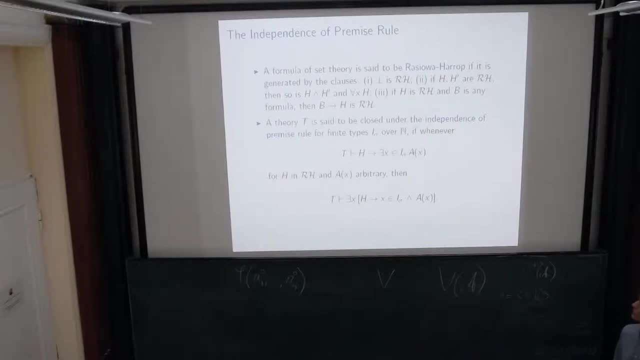 correct notion of realizability. oh, that's interesting. i haven't checked it. no, yeah, i think it's. since you mentioned q-realize, yeah, q-realizability is very prevalent in this area. i, i don't know, i, i this q-realizability, always feel a little bit uneasy. 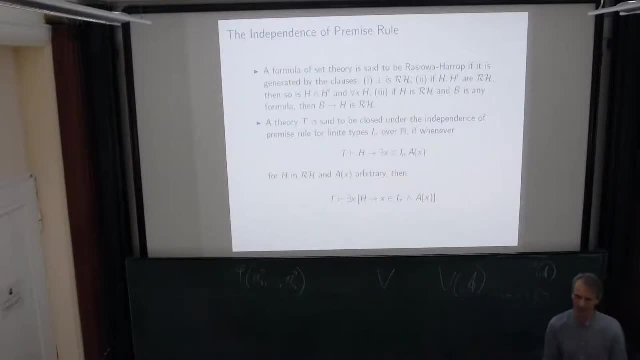 because it's not close under logical consequences. so that's why it's. it's not uneasy, it's still very useful. yeah, yeah, so sorry. my question should be formulated as follows: that in the in the equation x is in i, i sigma. can we move to the outside?